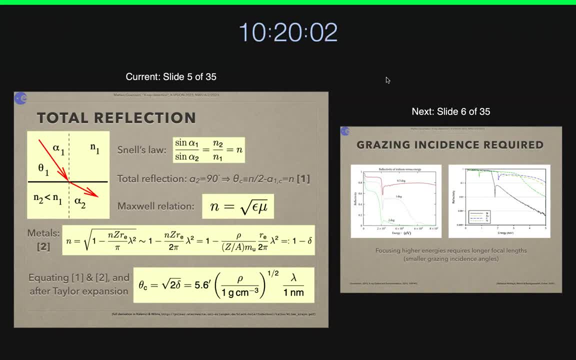 So we need to have a system which is able to reflect X-rays using the total reflection principle. And if you look at the basic physics of total reflection and if you put the numbers, the wavelengths, that corresponds to a typical X-ray photons which is of the order of tens of angstrom. 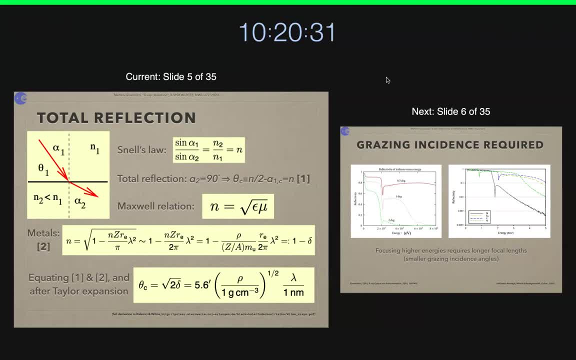 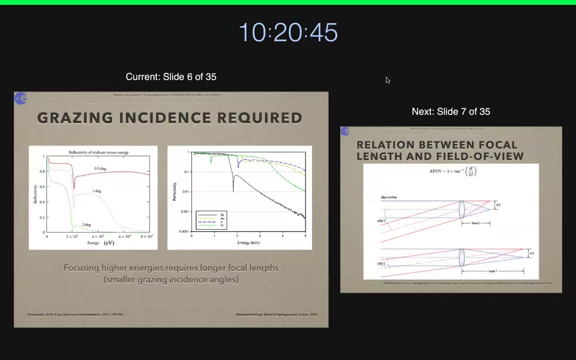 you immediately see that in order to achieve the reflection from a surface, from an optical surface, of X-ray photons, you need to have very low angles of influence. We call the talk of grazing incidence. Now. grazing incidence requires that you have to have an optical system. 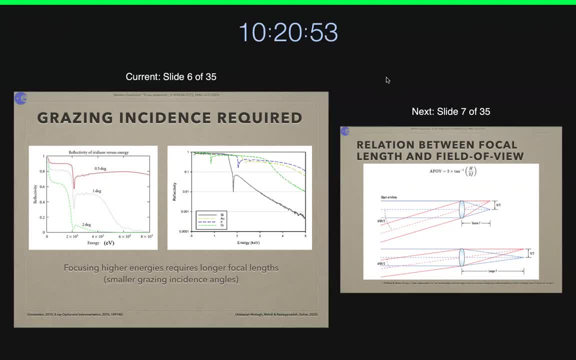 that essentially whose photons are hitting your reflecting surface as an angle which is essentially lower than one degrees, And the reflectivity is a strong function of the value of this angle. This is shown in the last slide. This is the left plot of this slide. 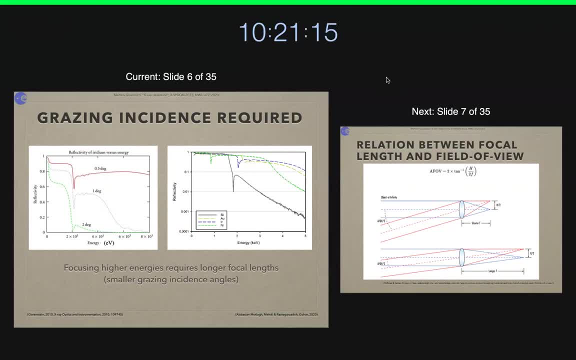 which shows as a function of energy. Be careful: The energy is essentially goes from zero to eight thousand electron volts, So eight keV, KeV, kiloelectron volts is essentially the basic units of energy that we use in X-ray astronomy. 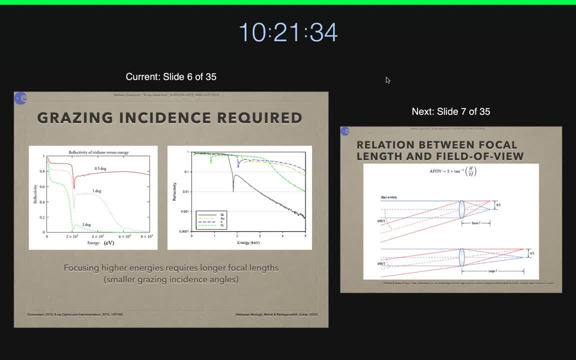 And this compares that the reflectivity of a surface covered with iridium, one of the elements which is mainly used for optics in X-ray astronomer, for different values of the incident angles: Two degrees, one degrees, 0.5 degrees. 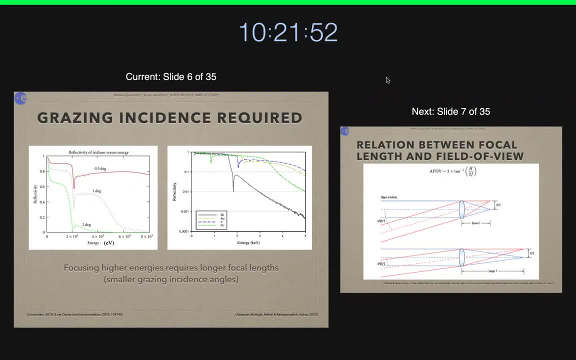 And you see the difference is enormous. So the more grazing incidence you need, the lower the grazing incidence, the higher your reflectivity. This has immediately a consequence. You will see that, you know, since if you have grazing incidence, you have a very low effective reflecting area. 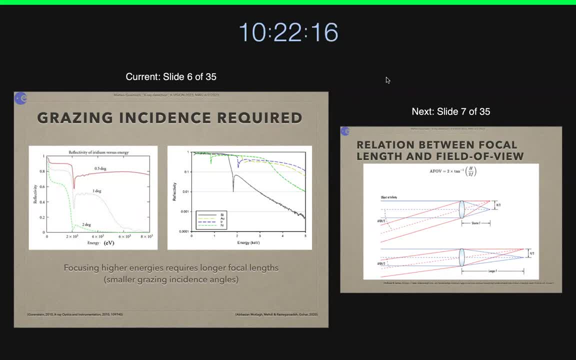 So that's why, if you look at an X-ray telescope, by variance with an optical telescope, you will see very often nested shells, because we want to enhance the reflective effective area that in each shell is relatively low, Or you create intelligent tricks to have multiple reflecting surface. 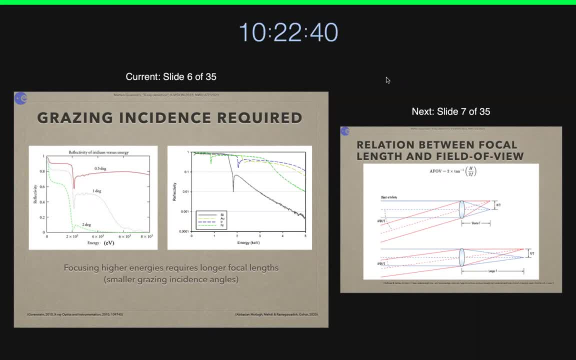 And that will be the subject, one of the subject of my last lectures on the future of X-ray astronomy. Another thing that you have to notice is that. Another thing that you have to notice is that That's me. that's me sorry. 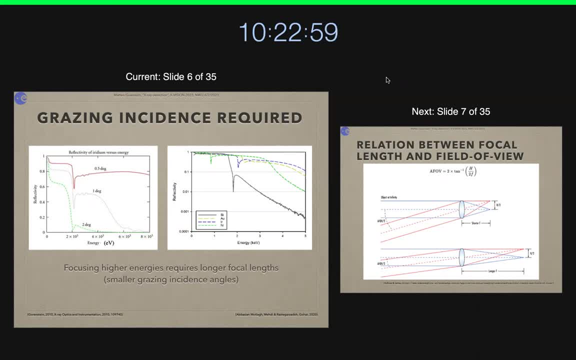 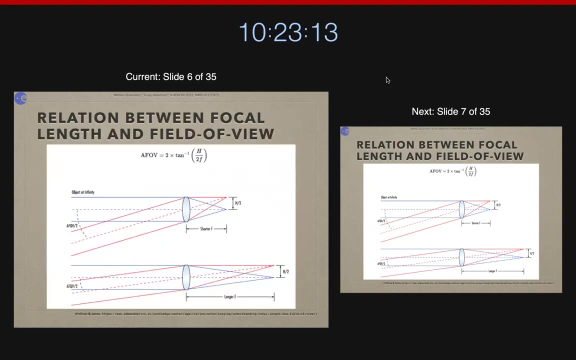 Focusing higher energies requires longer focal lengths. This is why one of the three missions we are going to deal with in these days has an extended boom, And I will leave you to guess which one it will be by the end of the day. There is also a relationship between the focal length. 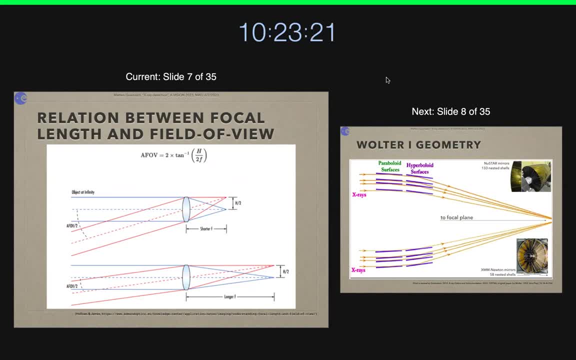 and the field of view. If you have a shorter field of view, a shorter focal length, you have a higher field of view. Correspondingly, if you have a longer focal length, you have a smaller field of view. So it's very difficult to have an instrument. 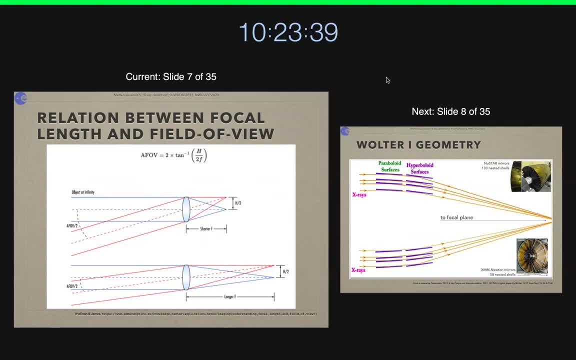 with high X-ray reflecting power- sorry, operational in the highest possible energy range where the focusing optic is possible, and survey capabilities. I'm sure that Christine is going to tell more about that in her presentation later today. Now, since the 60s. 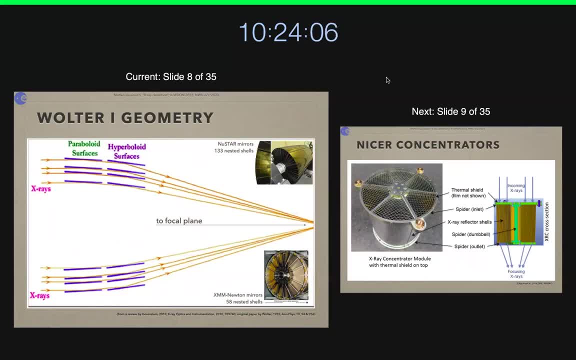 there is a sort of reference geometry that has been used in all X-ray telescopes to focus optics, which is the so-called Volter 1 geometry, which is a combination of a paraboloid surface and an hyperboloid surface, And this allows you to achieve 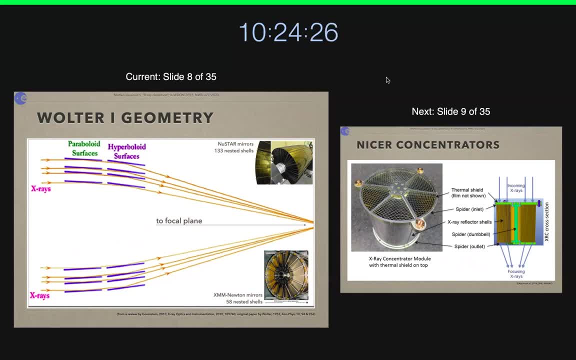 the best focusing power and also the best correction of optical aberration. Now there are different ways of implementing this kind of perfect geometry. There are conical approximations often used for the paraboloid surfaces, but these are by far and large. 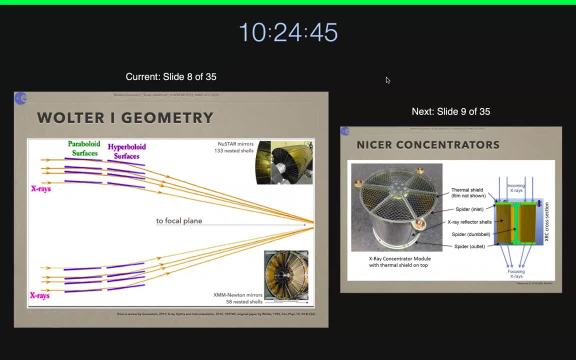 second-order technical details for you, But the important point is that, in reality, if you don't have very strict requirements on the quality of your image, you- actually the paraboloid surface- are sufficient for you to focus a light from a source at infinite. 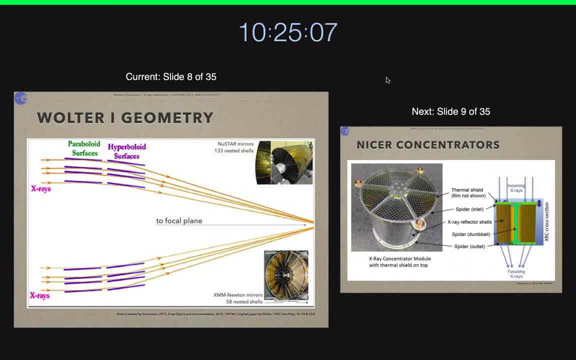 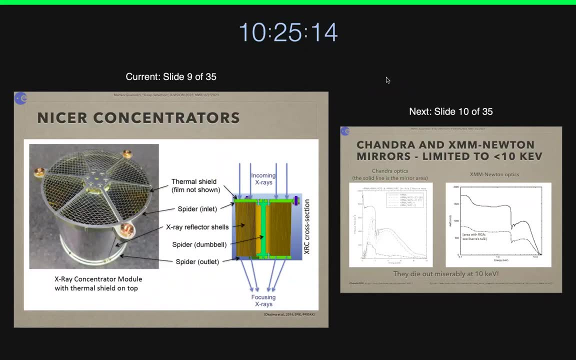 to the focal plane of your detector. So, in fact, an instrument like NICER that doesn't have strong requirements on the quality of the image because, as I show you later, essentially the NICER detectors are single-pixel detectors. 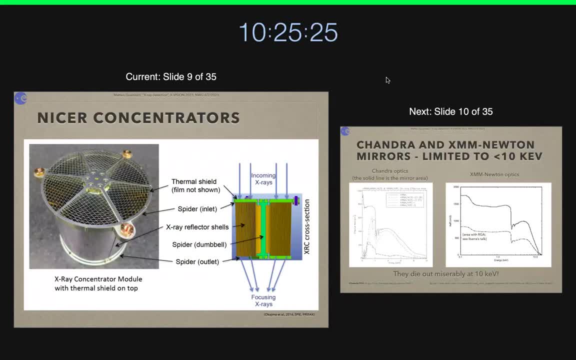 they can actually get rid of one of the stages and just having reflection by the paraboloidal surfaces, which make, of course, the technology of construction of these things much easier, Something that it will be all clear often to you in my last day presentation. 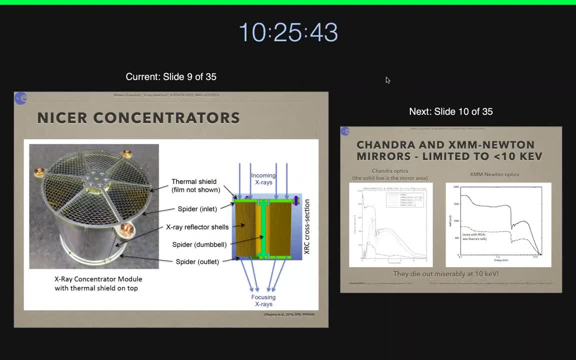 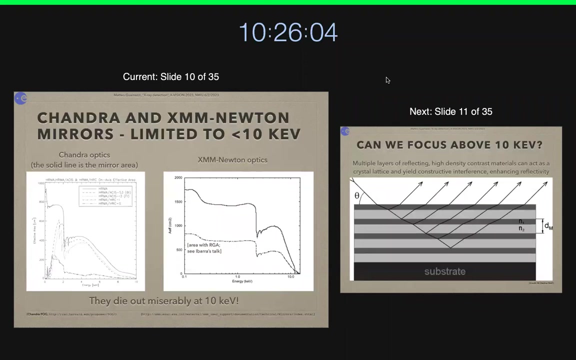 most of the technological achievements that we have obtained in space, in space science, are limited by money, So if you can do something cheaper, this is always welcome for every space scientist. Space agencies don't like wasting money Now in the history of X-ray astronomy. 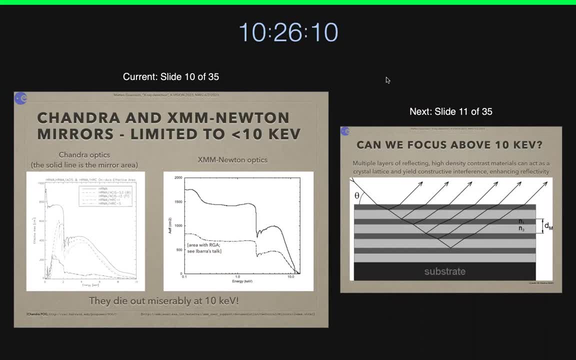 over basically half a century, has been limited, if you look at focusing measurements, to the 10 kV band. So we had optical imaging instruments, you know, focusing telescopes, since the 80s probably, but none of them was able. 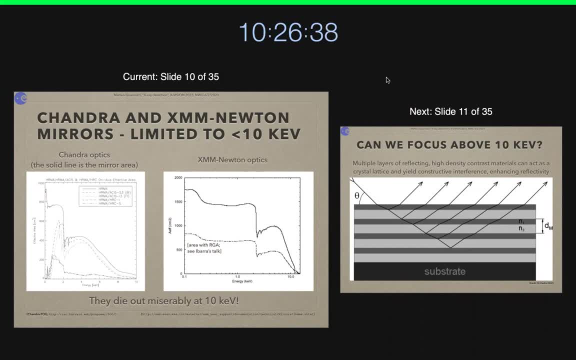 to have sufficient collective area above 10 kV. This is when a great deal of the science in X-ray astronomy was done below 10 kV, until a pivotal moment in the history of X-ray astronomy, when NuSTAR was launched. Now it's fair to say. 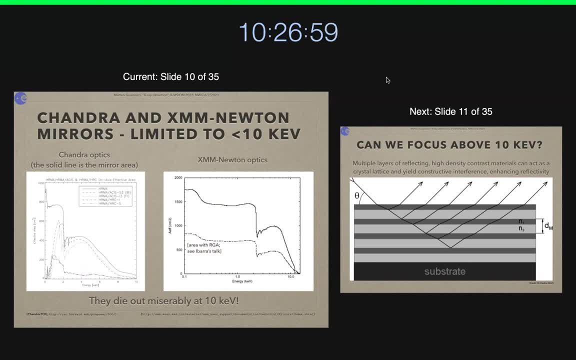 as it will be clear from the science presentations that this is also the wavelength until 6,, 7, 8 kV, where you have the strongest atomic emission and absorption lines in X-ray plasma. So you know, there was a nice match. 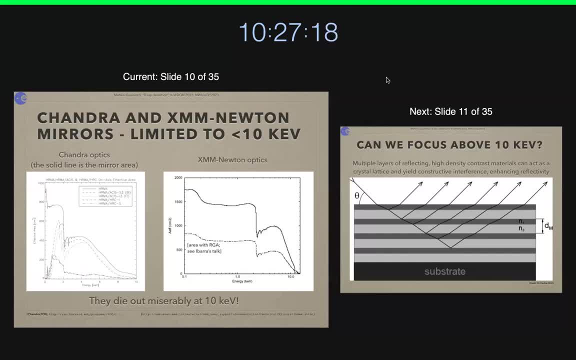 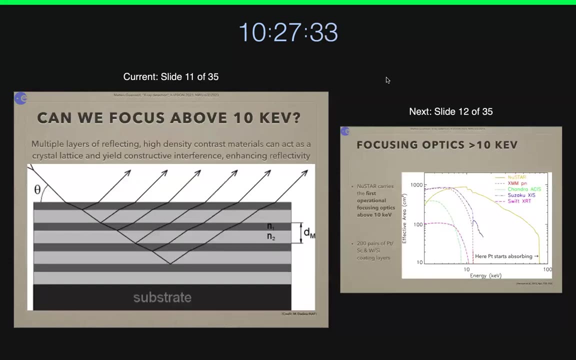 between technological capabilities and science requirements. But, as Christy is going to say, surely later today or tomorrow there are plenty of new science that focusing optics above 10 kV could have opened and did open when for the first time, the technical of multi layers 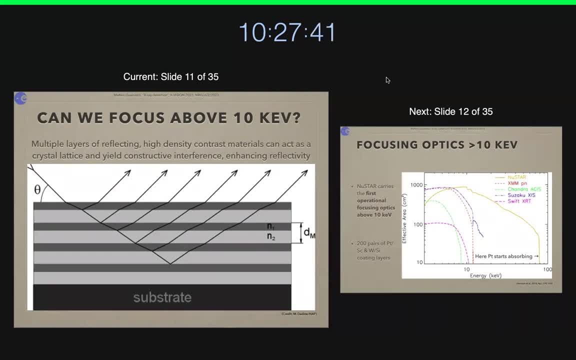 multi layers of reflecting matter was implemented in space. The trick is, if I have lots of the you know layers of materials that are able to reflect the light, I can in a sense- you know- accommodate, I can create a trick. 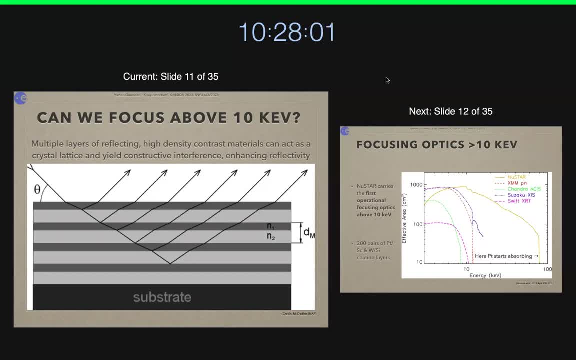 where I increase my effective area by creating constructive interference among the reflection of these layers. That was the trick that was used in NuSTAR in order to enhance reflectivity above 10 kV and achieve an effective area which, you know you can't even compare with. 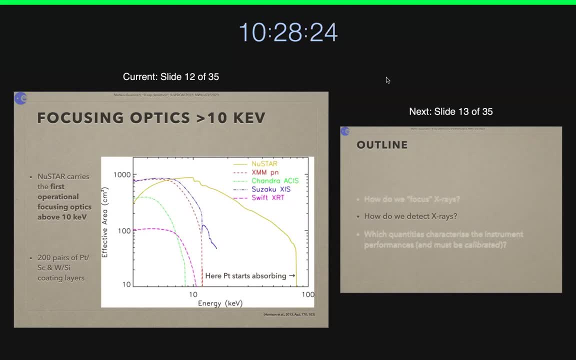 Chandra XMM, with Suzaku, with ASCA, with Bepo-Sachs, you know, with all the instruments, and Bepo-Sachs didn't have optics that were flying X-ray optics before that. So this is a plot. 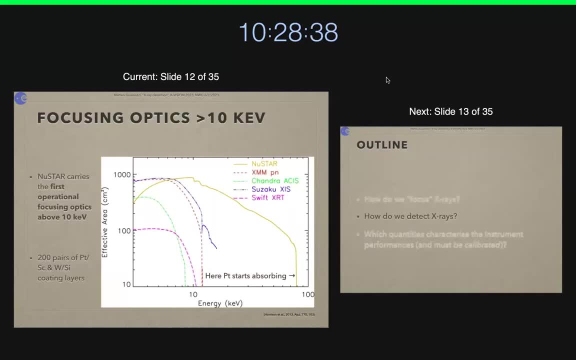 one of the plots that you have to get familiar with On the y-axis is a quantity called effective area, which has the unit of an area. It's not the geometrical area of the optics, but it's a quantity that takes into account. 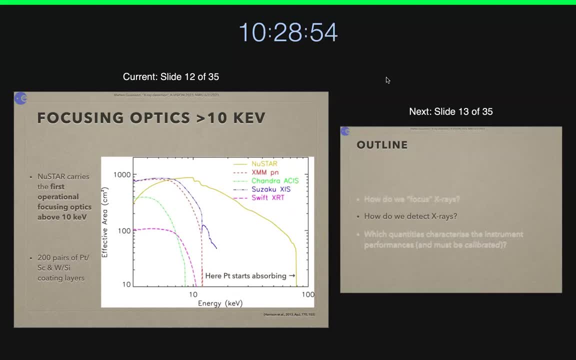 all the components that eventually make up the capability of an instrument plus optics. optics plus detector and instrument to detect X-ray photons as a function of energy. And the orange line is NuSTAR compared to you know all the active and still active instruments. 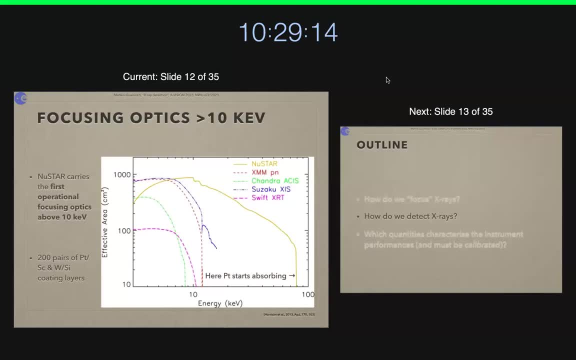 at that time, except Suzaku, with optics, so with focusing optics, And you know, there is, of course, no comparison in the range above 10 kV Now, something that I'm not stressing. why I'm so, you know. 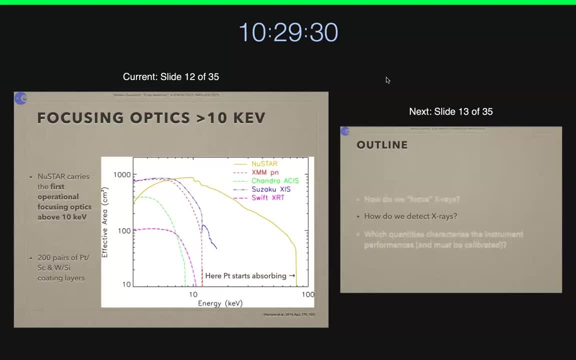 why I'm stressing so far the concept of optics. People say: well, you know there are several ways of you know how detecting. you know you have detectors in X-rays. Can't you simply put your detector in, you know? 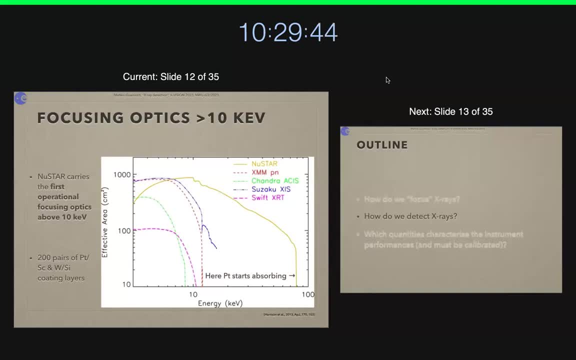 looking at the sky and see what happens. Why do you want to focus Now? just to make sure? I think this is a trivial question for most of you, but optics, focusing optics, is the key way in order. first of all, 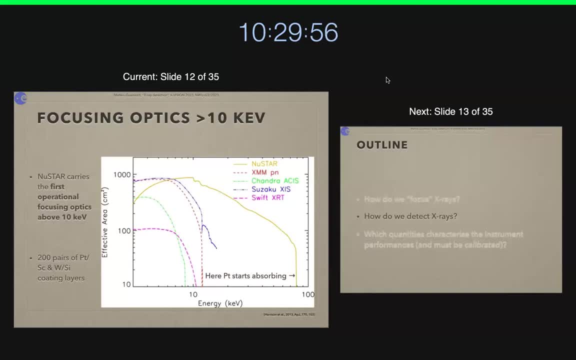 to do images that allows you spatially resolved analysis of diffuse structure in the sky And you will see there are many objects in the sky that are diffuse, that are extended, large-scale structure, and if you don't have optics you can't really understand. 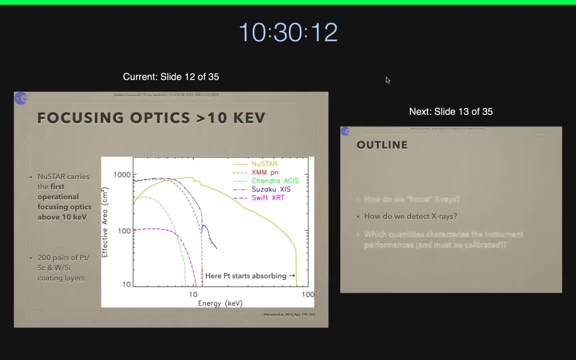 what's happening in them: Sofernova, remnant galaxy cluster, galaxy groups, all these kinds of stuff. I work in Asia, And but there is a more fundamental reason why you want to focus. The reason is that, if you are able, 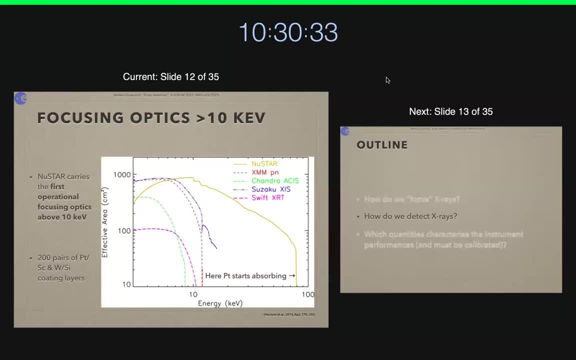 to concentrate your photons in a small region of your detector, you are enormously increasing your signal to noise. You reduce the background underlying your source. The background is always the first order proportional to the volume of your detector. So if you just put the concentrate detector in space, 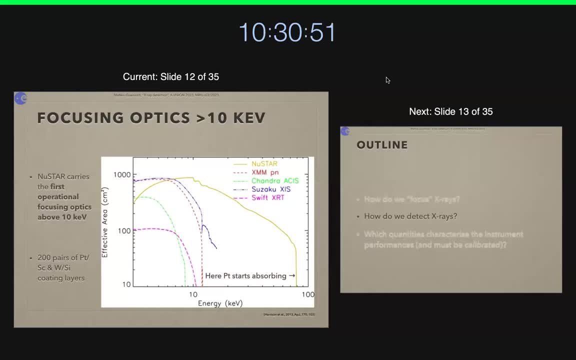 and you tell me all the photons that you see, you will get lots of background photons you're not interested in, proportional to the volume of the detector, and it will be very difficult to get a nice signal to noise. By focusing you actually get. 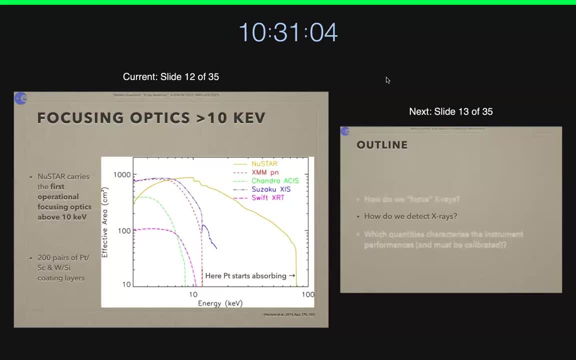 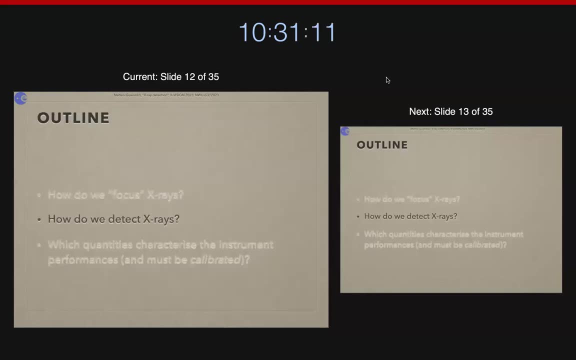 the best ratio between the source you are interested in and the background photons you just want to get rid of. So how do we detect X-rays? Well, fundamentally, the process that you are using is photoelectric absorption. I show here two X-rays. 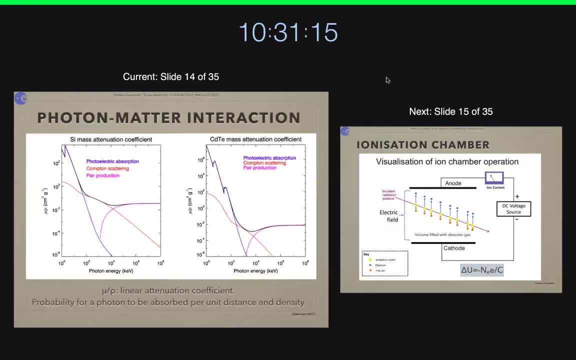 that you can see in the background. The first one is the X-ray that you see in the background. The second one is the X-ray that you see in the background. I show here two plots: as a function of energy, of the attenuation coefficient for two materials. 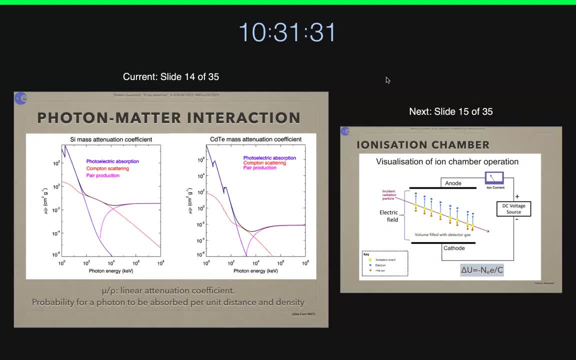 silicon and cadmium tellurium. The reason why I've chosen these two elements will be clear in a moment Now. be careful now at the X-ray, at the X-axis units. in this case These are kiloelectron volts directly. 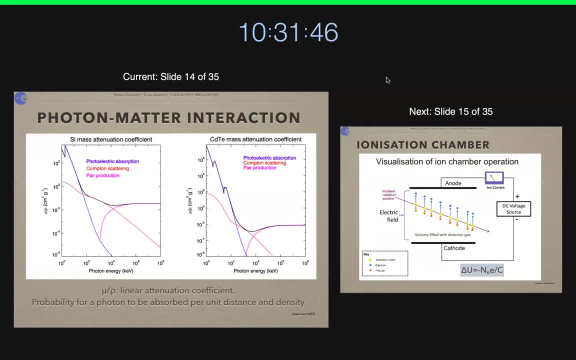 So, since you know nu star and XMN, they go up to 10 Chevy, nu star goes up to 70 Chevy. What you are actually looking in both plots is just the left part of the plot. That's where the instruments. 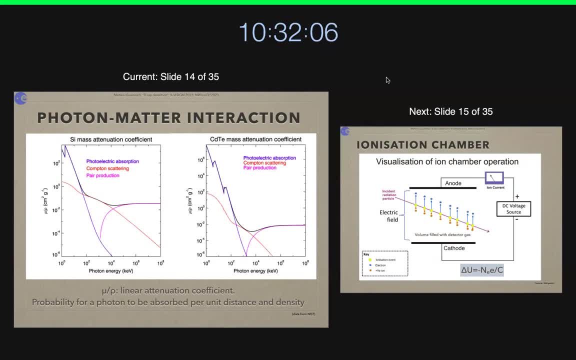 are effective and where is photoelectric absorption dominates. So we need to add detector capable of using the photoelectric absorption to create quantities that can tell us that the photon is interacted with our detector and maybe that we can also derive the energy of the photon. 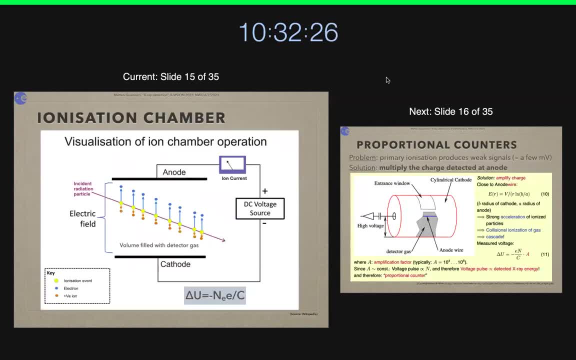 with which? energy and when? Now, the simplest concept that since the beginning of X-ray astronomy has been simply ionization chamber. So an incident particle is coming, it's filled with a certain type of gas, typically, you know, relatively inert gas. 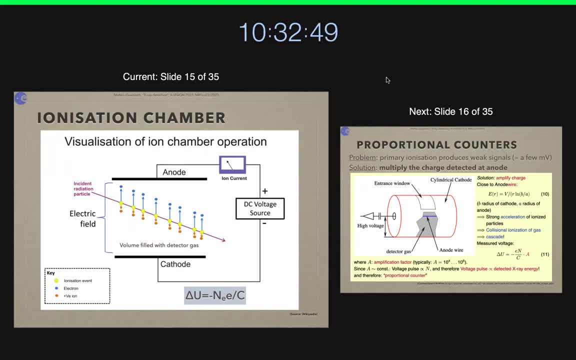 and it creates a track, a ionizing track, and positive ions remains left after the electrons has been ejected, And then, if you put an electric field within this gas, you can essentially collect the electrons that have been produced by this interaction track and there is 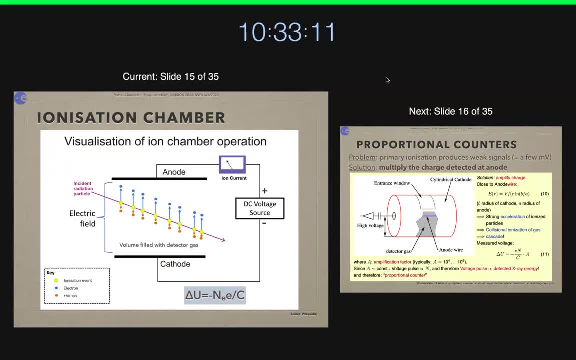 a sort of proportionality between the number of electrons or the current that you measure and the energy of incident photons. you can reconstruct the energy in this scheme. There is no mention. I've not mentioned at all where the event happened. Event can happen. 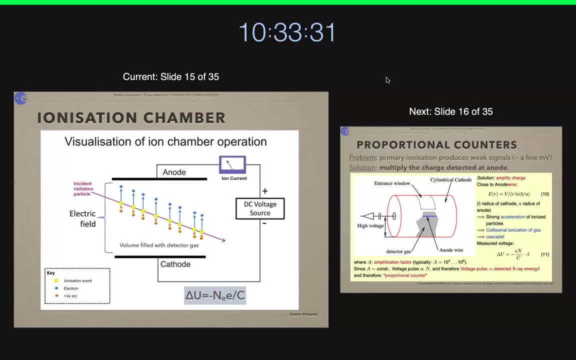 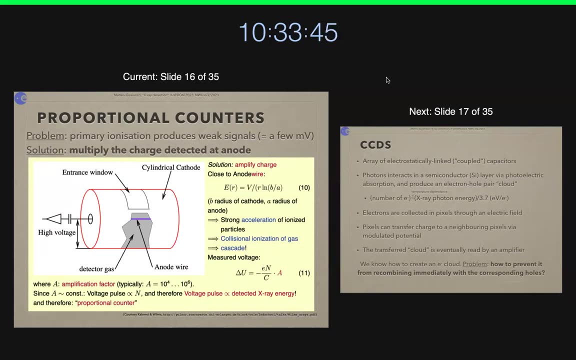 in everywhere in the camera and this kind of very simple concept does not allow you to have a very accurate positional reconstruction of the events. But the problem with this scheme is that the um, the, this primary ionization, produce very weak signals that are 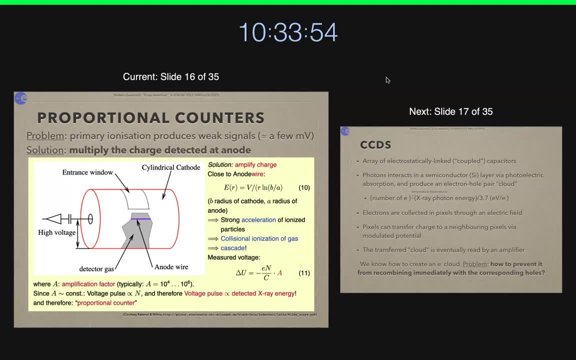 very difficult to detect. So typically these ionization chambers were coupled with proportional, with sorry, with um uh, with um systems, electrical systems capable of amplifying the charge when the charge was red, In order to get an amplification. 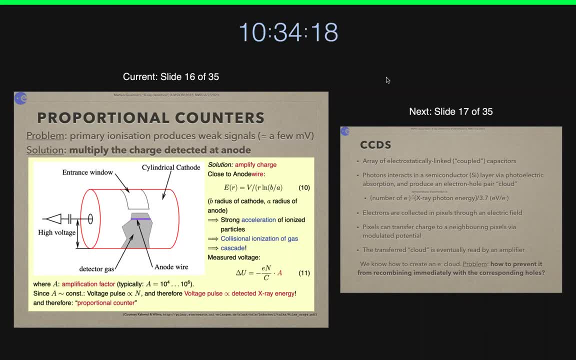 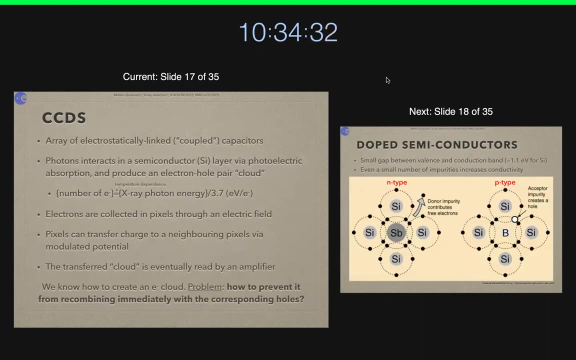 factor of the order of hundreds thousands. this very simple concept has been the workhorse of X-ray astronomers for decades. But the great you know, the big jump ahead was when X-rays, the CCDs, were used, and for the first time. 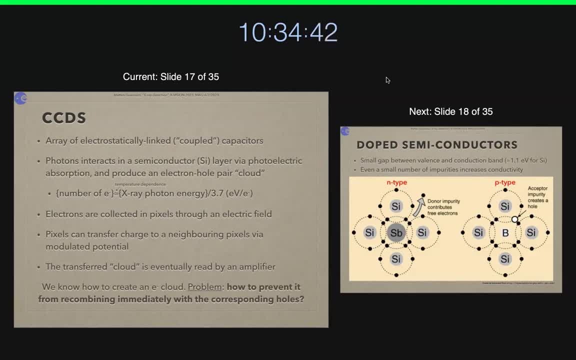 they were used on a Japanese led satellite called ASCA in the middle of the 90s. Now CCDs are, you know, we have in all of our digital device, but they are of course optical CCD. So there are some. 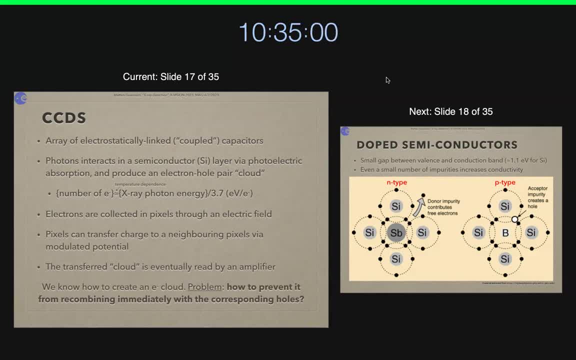 difference between the way optical CCDs works. and well, of course you are familiar, if you are a real astronomers, to the CCD in optical astronomy. but you know there are certain difference, important difference, in the way X-ray CCDs are used. 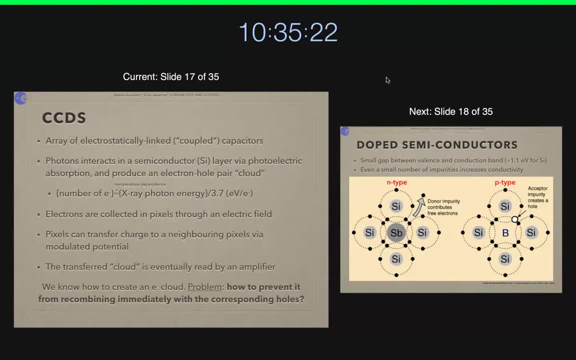 So the first thing that we are going to do is to measure the energy of the incoming photons. So what we are going to do is to measure the energy of the incoming photons. So, if I am able to measure accurately the energy of the 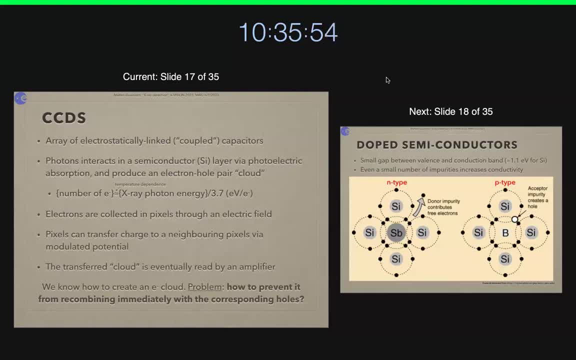 event as produced, I can very accurately reconstruct the energy of the event. But CCDs do also something more for you. I can organize the CCDs in pixels, And so if I know in which pixel a certain event has happened and I know. 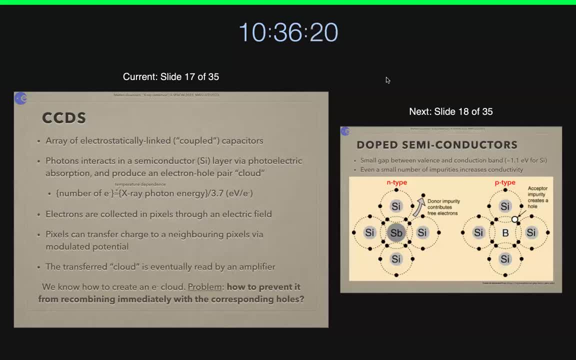 where my telescope is, I can exactly pinpoint where the event happened. So I can do accurate imaging reconstruction Now, once the event happens in a given pixel of your semiconductor. you know they are of a little use of these electrons through a. 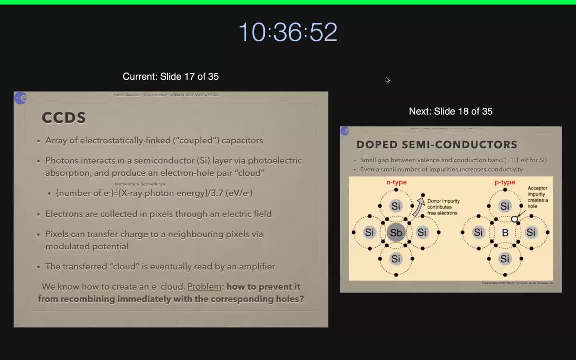 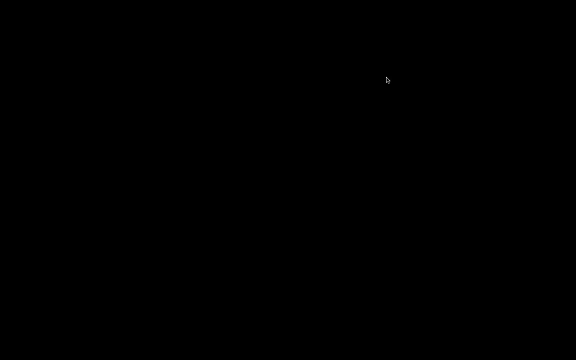 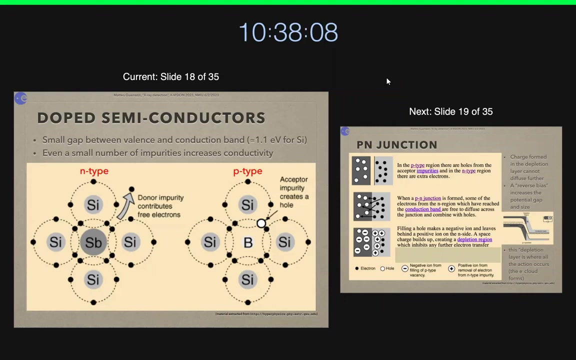 row through a column, up to the point where there is a reading system, an amplifier that is able to read the number of holes. So you know, the tendency would be to recombine very quickly. So you have to manipulate the semiconductor. 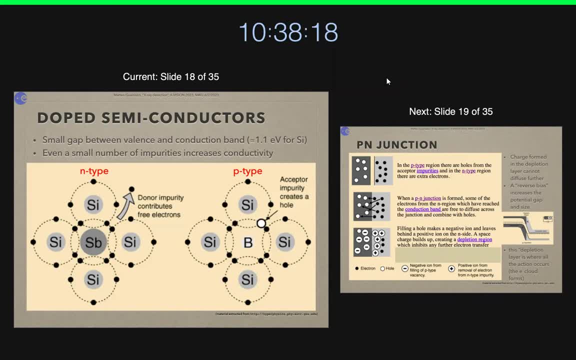 in certain special way. Essentially, we have to add sometimes some impurities that essentially create, in a stable way, an excess of negative charge electrons and regions that have an excess of positive charge holes or positively ionized ions. The first, the lot of the 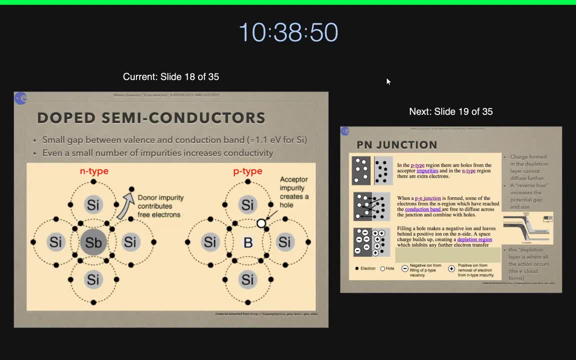 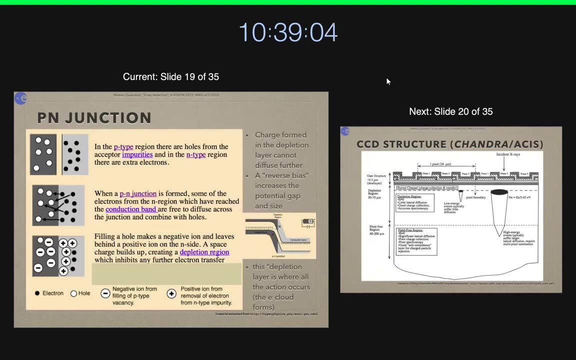 former are called n-type and the latter are called p-type- Yeah, for lack of a better name. And now, if you join them, okay, at the junction free electrons, they find their friends, their holes and they recombine. 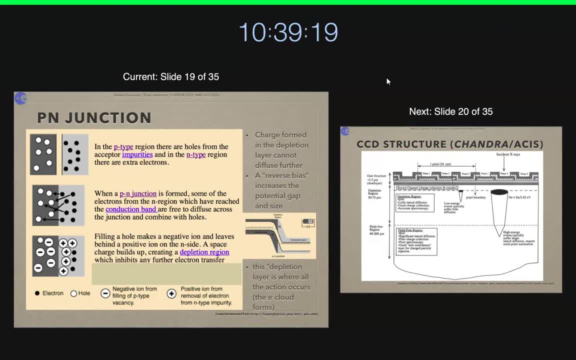 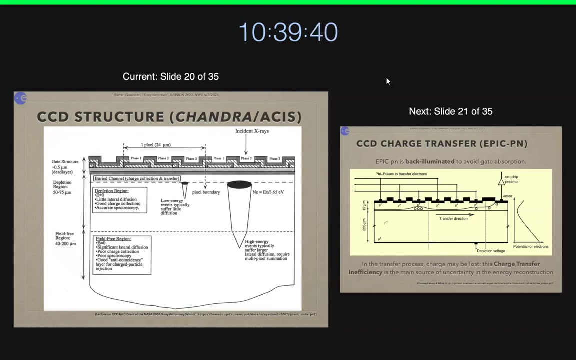 And this creates a layer of positive and negative charge that prevents electrons and holes outside the system, which is enhanced by applying appropriate voltage to the system, which is where actually the detection of the stray photons happens. So this is a scheme. 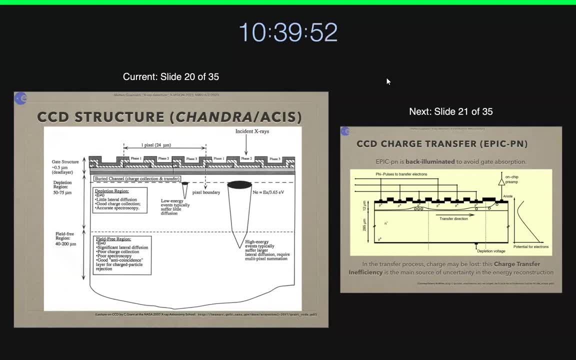 a conceptual scheme of a CCD structure in Chandra for the diffusion of the very little lateral diffusion of the charge, And therefore, once the charge is concentrated very well on the pixel. Now, of course, there are also events that are so energetic. 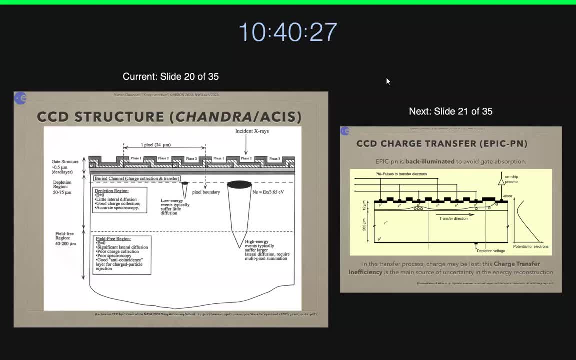 that can go very far. So what we have to do in X-ray astronomy is that, while ideally we would like all our events to happen in a given pixel- because one pixel means one position in the sky- this almost never happens. 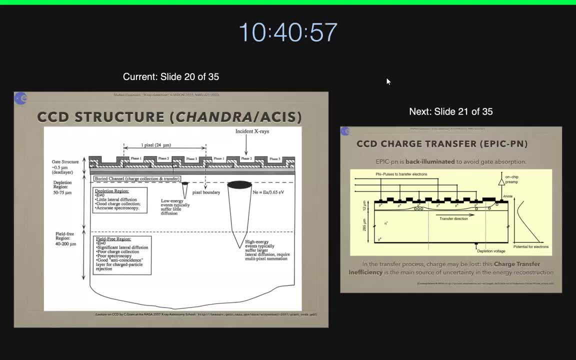 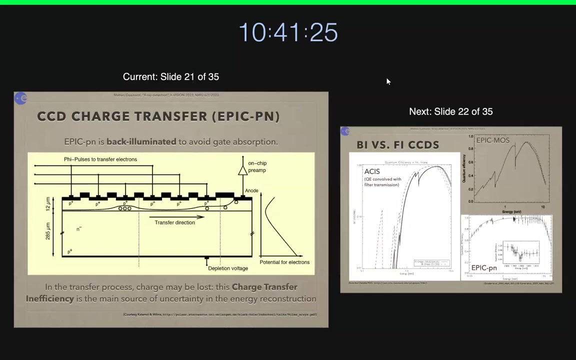 Most of our events have the structure of different pixels that they all belong to the same event, which is the total energy of the event. You immediately see that if a certain event creates a signal in various pixels, the signal is the signal of the event. 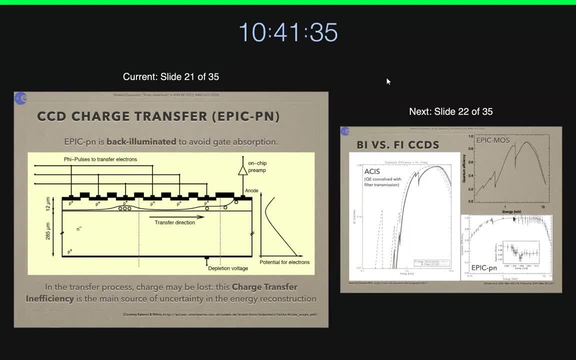 So this is something that I have to deal with via data analysis later. From the point of view of the physics, I have my cloud of electrons and I am transferring the charge from the position where it was created- the cloud, to the amplifier. 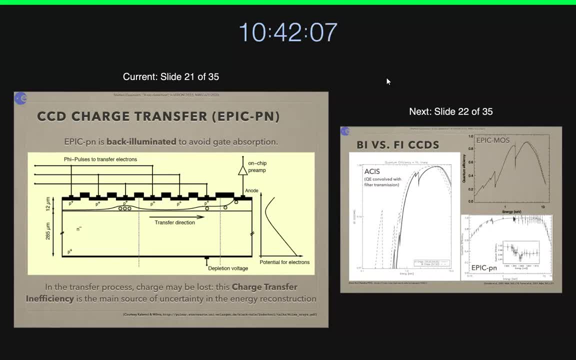 to the reading node does not come for free. You may lose electrons over this process. In fact, you lose electrons over this process And you lose a high number of electrons. So some optical photons create basically one electron, And so 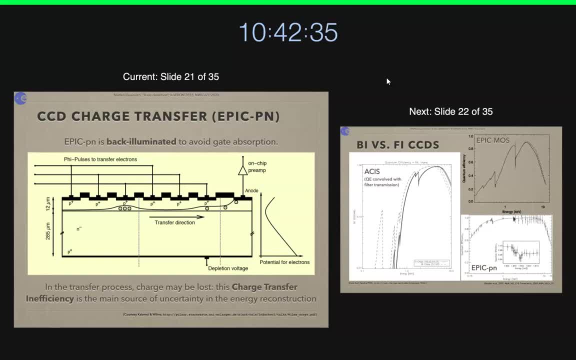 in fact that's the reason why you work essentially most optical CCD in frame accumulation mode, But in the case of X-ray astronomy each event creates thousands of photons of 60 kV. It's creating almost 2,000 events. So 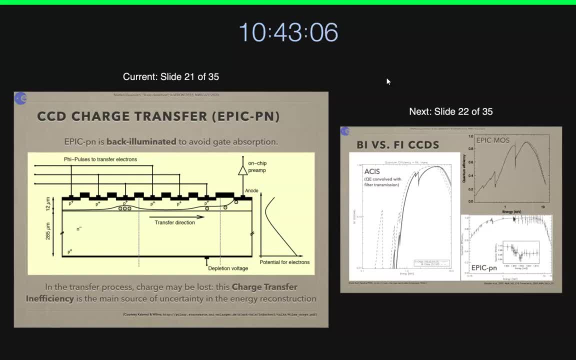 even if I lose 10 to the minus 5 events for each step of my transfer. but my system has thousands of electrons. in a CCD like the, This is a very important phenomenon. You see what the risk is. I read a certain number. 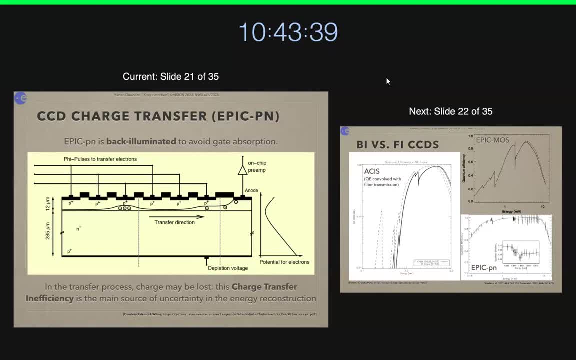 of electrons, and I say the energy number of electrons times 3.7 eV. But that's not true, because the energy is very low. So I can see that the energy is very low. So I can see that the energy is. 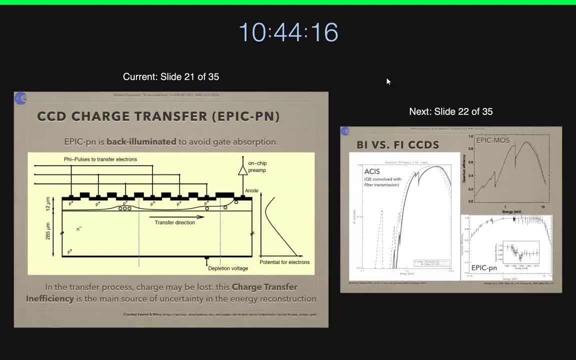 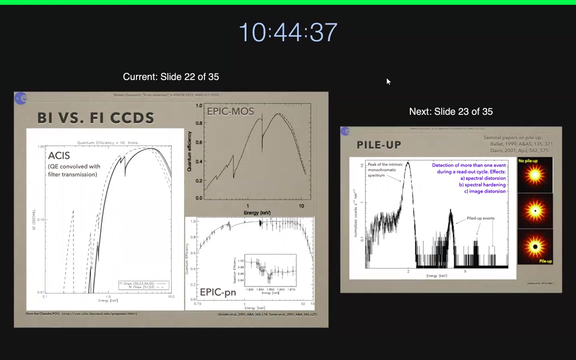 very low And I can see that the energy is coming from above, which means that some of the photons actually never reach the depletion region of the CCD. They are absorbed by the gate structure of the cell. So I can see that the energy 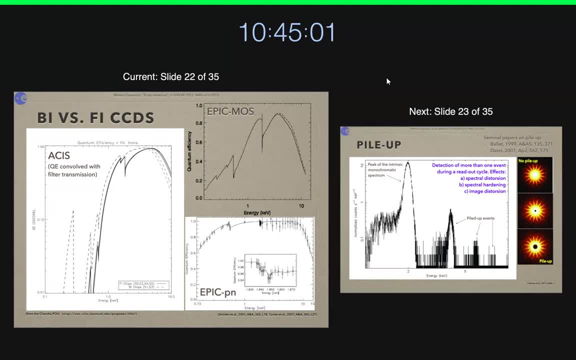 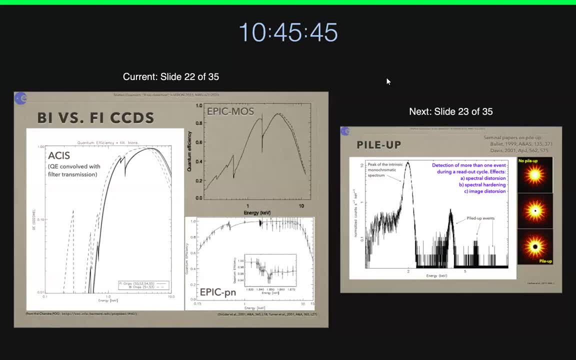 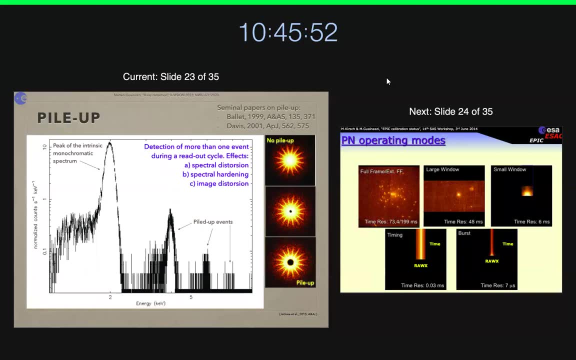 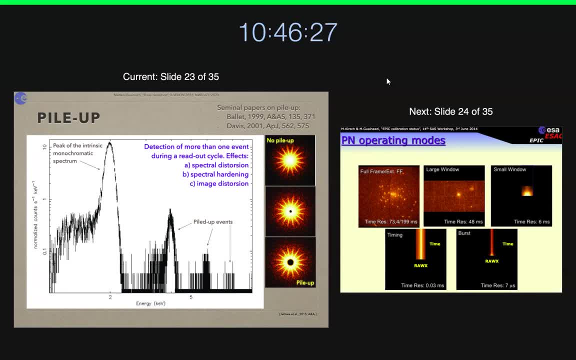 can see that the energy is very low. So I can see that the energy is very low, So I can. And the system doesn't know by itself that these electrons have been created by two events simultaneously hitting the CCB. Simultaneously means within the same accumulated interval. 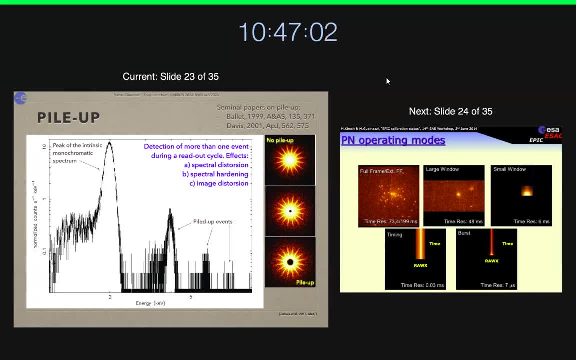 And this creates a phenomenon which is called PILUP. PILUP has two effects. First of all, it makes you calculate the wrong plot, Because you believe that a certain number of electrons have been created by one photon, but they've been created by two photons or three. 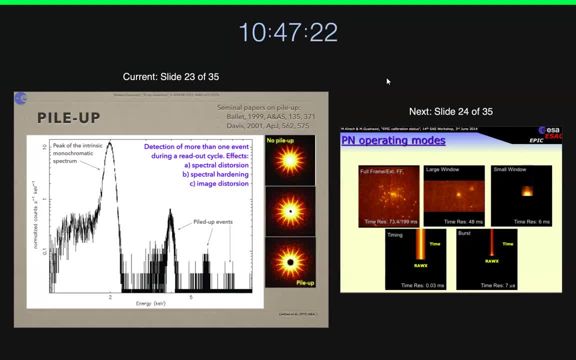 Therefore, your plot is wrong: actually lower. You believe that less photons are being detected than in reality. But there is a second, the most more important effect, which is spectral distortion. If I detect several photons At the same time and I just measure the collective cloud, the collective number of electrons, 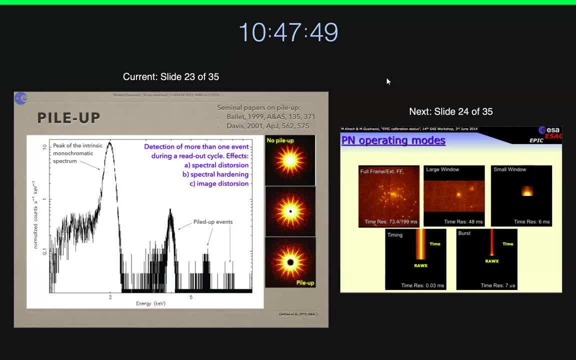 Generated by any events. I will sum up the energy of individual events. So instead of getting a spectrum of, say, three events of energy one kV, I will get one event of energy- three kV. So I have less plot but a harder plot. 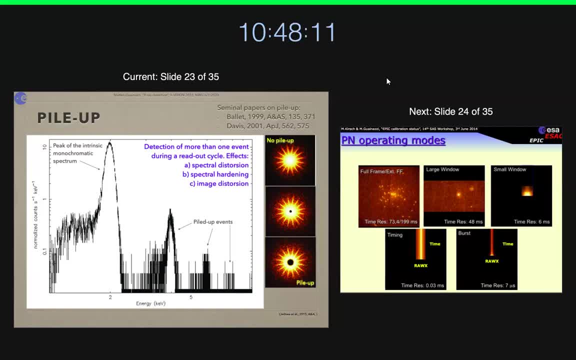 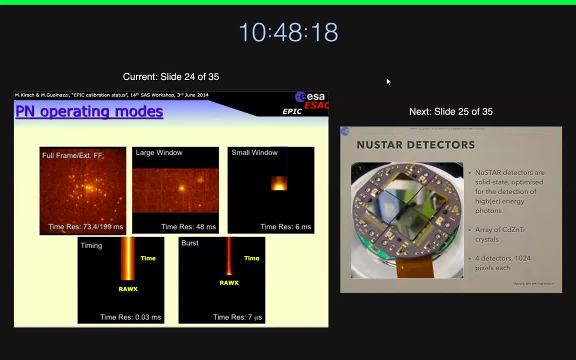 And PILUP is a true problem, As Hytor is going to show you for the XMM case very soon. The best way is to avoid PILUP, And avoiding PILUP is the main reason why the XMM use of EPIC instruments. 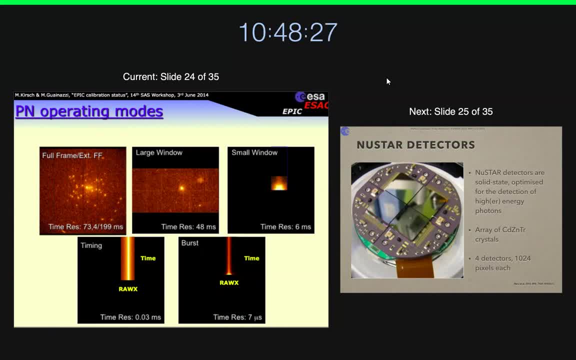 They have different operational modes. Sometimes we image the whole field of view, That is, the field of view that you know covered by our detector. In the case of the EPIC-PN, as shown here, it's 30 degrees, 30 degrees. 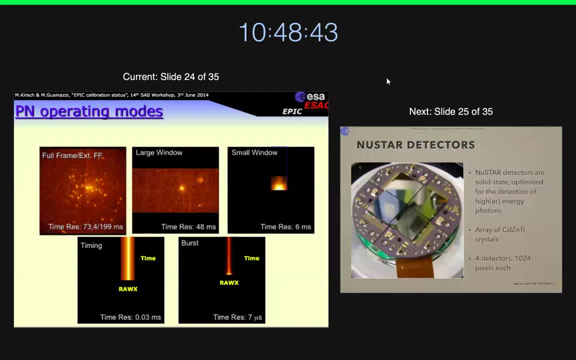 park minutes times, 30 days. But if you lose, if you look at the smaller region of the sky, you can read your UFO pattern And if I can read I can deal resources with a kind higher p12 on it without files. And that's why we add the large windows, small windows and even modes where you don't create images any longer. 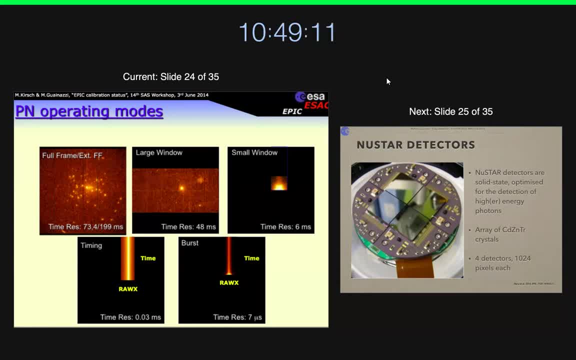 Where you don't create images any longer, accumulating photons, but you lose completely the information of where the events are lost. It is the price you pay for special timing modes that will actually have no imaging capability. Now we talked a lot about CCD. 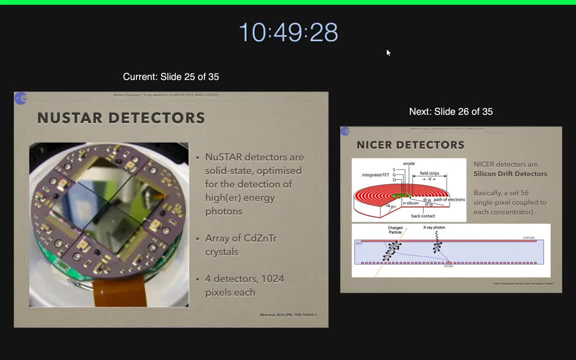 that are the instruments on XMM-Newton. NuSTAR doesn't have CCDs as such, but a solid-state detector. It's an array of cadmium, circonsium, circonium, tellurium crystals, zinc telluride. 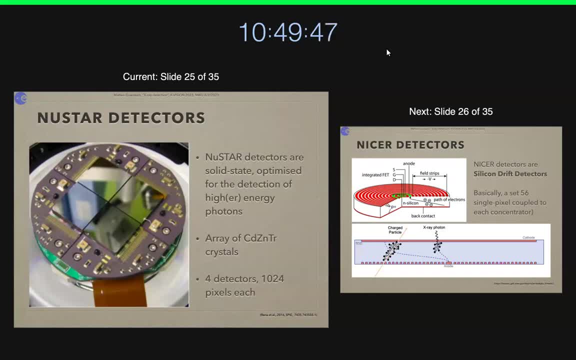 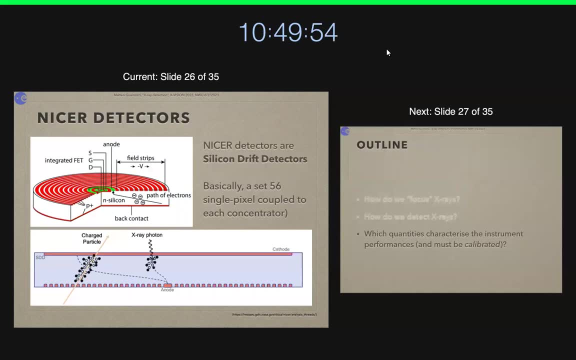 crystals. Okay, good, Thank you. And of course, since I know very little of them, I leave Kristen to talk about that. And also, nicer detectors are silicon-drink detectors. Basically, they are 56 single-pixel detectors each of. 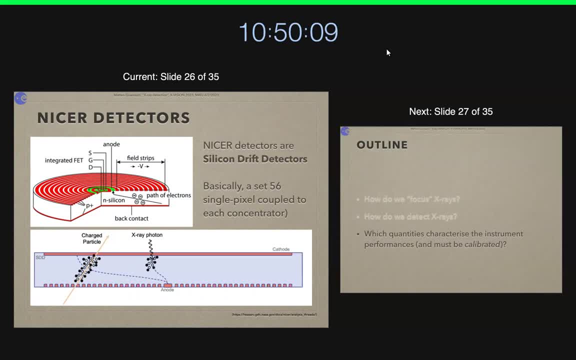 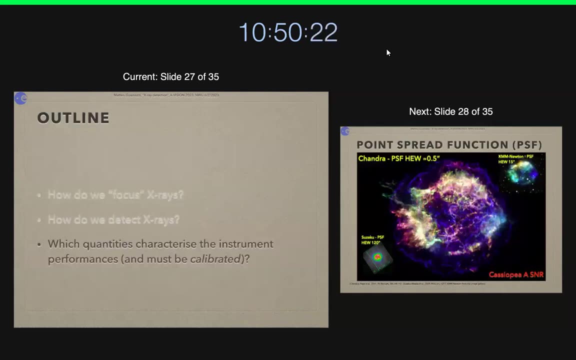 them coupled to a concentrator, And that's you know. remember I mentioned that a concentrator is no imaging capability, imaging requirement associated with NICER, essentially for this reason. Now, that's now the point where it comes, it comes. 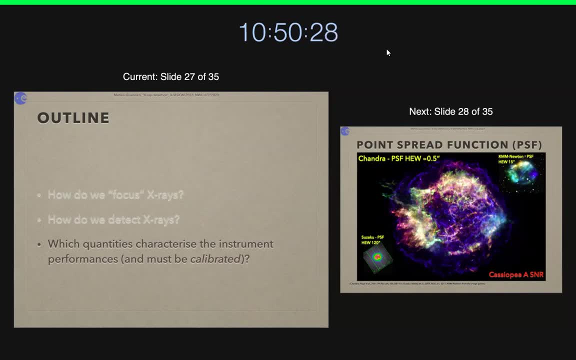 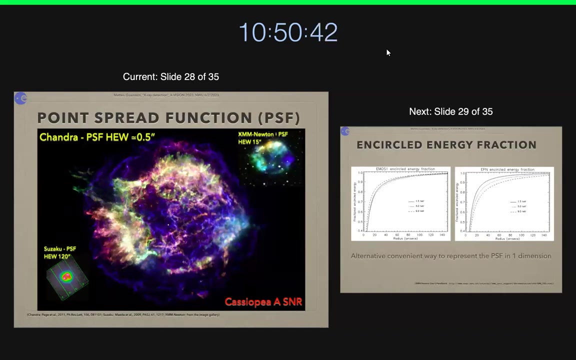 the point where you have to concentrate more because these are quantities. I'm going to show you the few quantities that you needed to get familiar with since the very beginning. The easiest probably for you to you know, get hold on when you have experience trial. 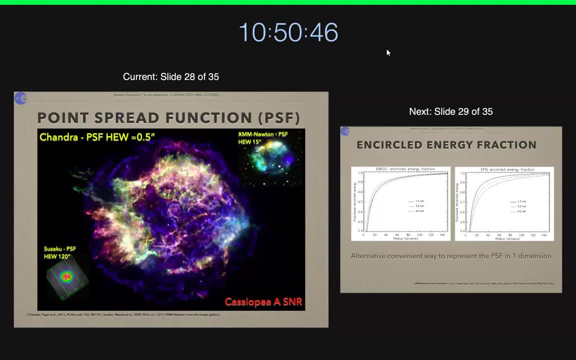 experience with astronomy and other wavelengths is the points-per-function, So it's the quality of your imaging. Points-per-function is the shape of a point-like source at infinite in your detector plus telescope system, And the big image is what you can get with Chandra, Chandra. 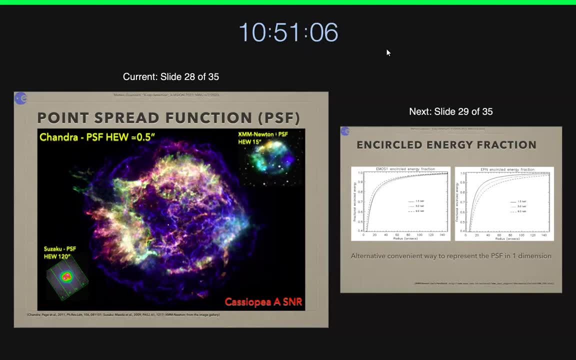 as you probably know, has the best image holding telescope current currently in operation, with a half energy width of the order of half arc seconds, And half energy width is the width of this image of a point-like source at infinite, where the you have. 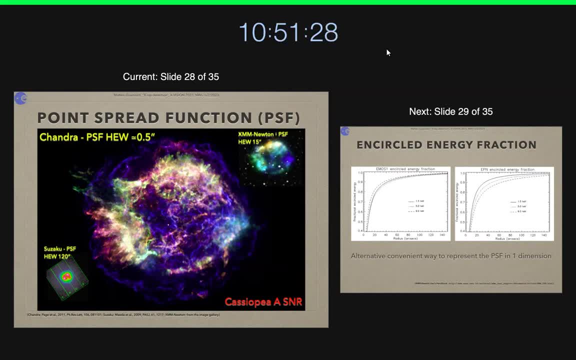 half of this energy, half of your events are collected, And I compare it with the points-per-function of XMN Newton in the top right corner, and an instrument with an even lower resolution solution which is representative of the type of optics that JAXA, the Japanese Space Agency. 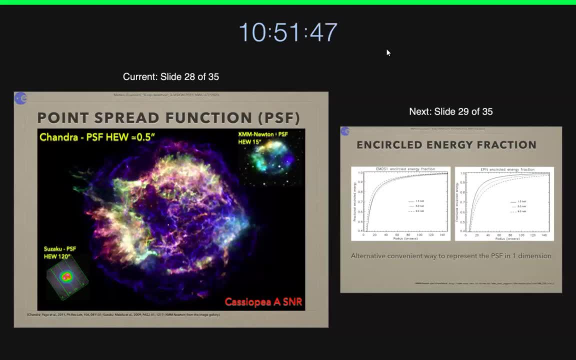 actually they are. American. optics is the goddard that the Japanese mission typically carry And you immediately see. of course you know that's an image that tells more than 1,000 words, but that's why Chandra is the. 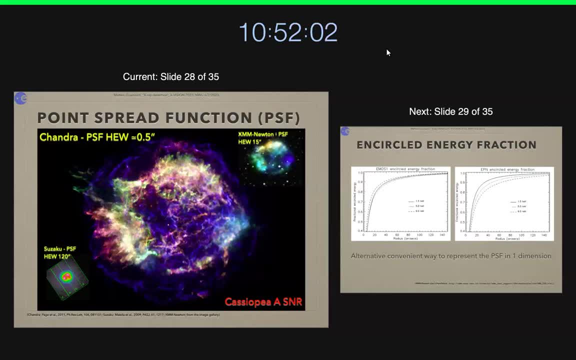 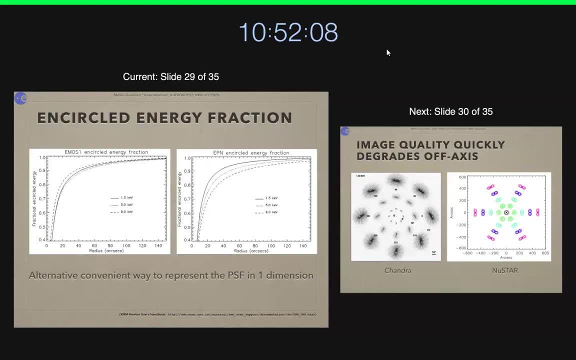 workhorse if you want to do very detailed X-ray imaging, energy dependent X-ray imaging of your source. But maybe more important for you to get familiar with is the encircle energy fraction quantity, which is an alternative, convenient way to represent the points-per-function in one. 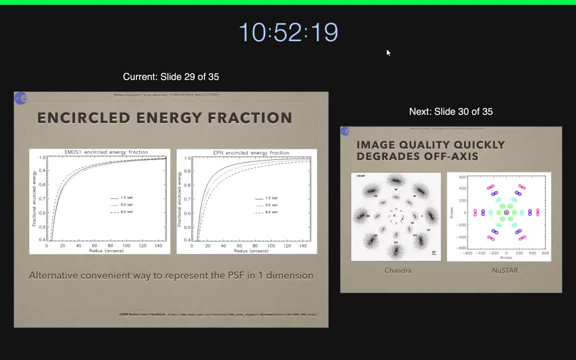 dimension. Essentially, the X-axis is radius and the Y-axis is the fraction of photons accumulated within that radius. And these are the encircle energy fractions for XMN Newton, from which you see that you know half of the energy it's. 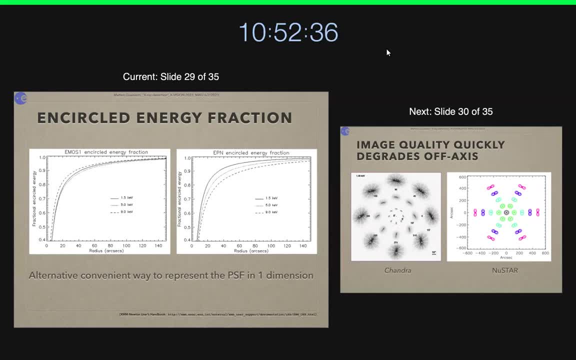 0.5 level is around 15 arc seconds. you see, in both cases There are small differences related to the quality of the mirror and also to the pixelization of the instruments, Now something that, if you work with XMN- 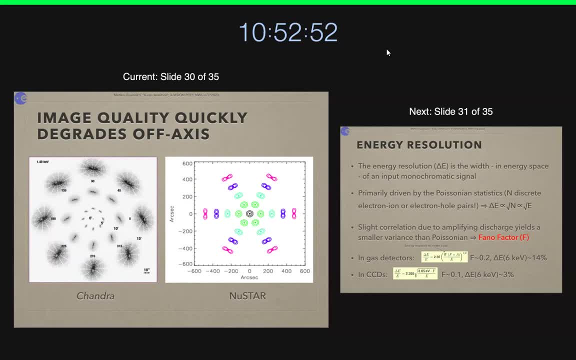 Newton, you should be dramatically aware of, but also if you work with this type, is that these are the numbers of the PSF at the center of the field of view, or, better said, where your optical axis is located, But the PSF the image quality. 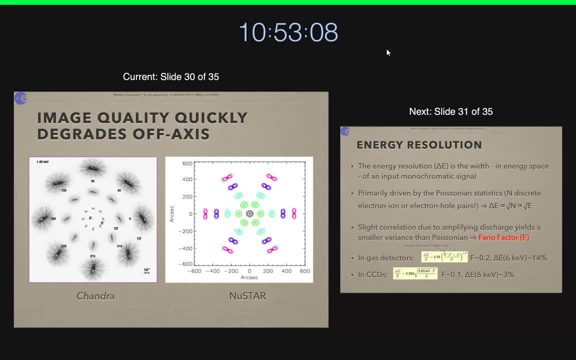 in X-ray astronomy degrades dramatically of axes. It happens for XMM. I've shown here the example of Chandra because you know Chandra has a point-track function better than one, except in the axis, If you go at the edges of the field of. 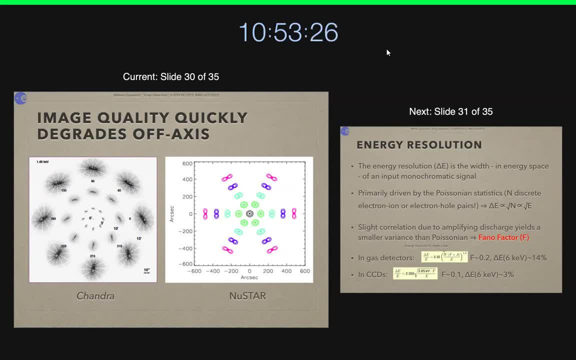 view, you get actually point-track functions that are significantly worse than XMN, Newton. The degradation of axes is very extreme And the same kind of degradation happens in the star. but more than the degradation in terms of, you know, quality is the fact that point-track 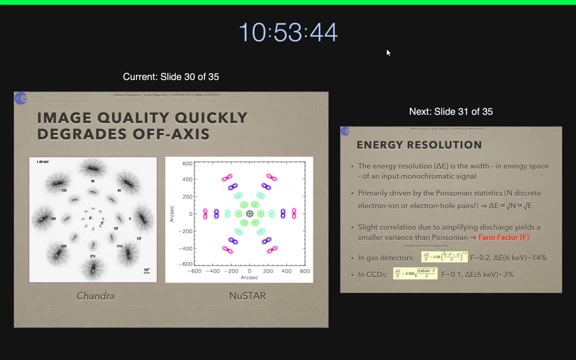 functions are steadily distorted. They are no longer nice radially symmetric, azimutally symmetric shapes. So this means that if you want to analyze extended sources which are very off-axis, in XMM for instance, that's searching for lots of troubles. 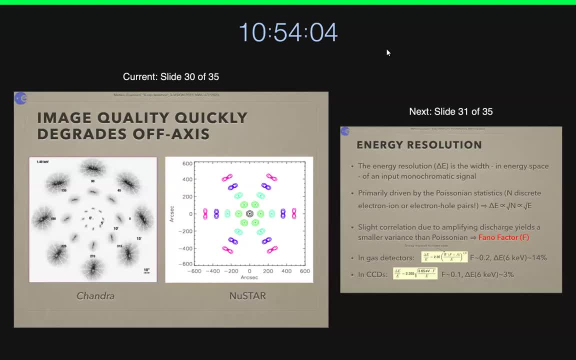 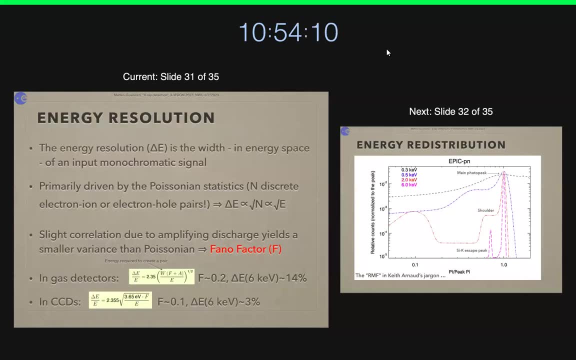 It's not an unsolvable problem, but it's a difficult problem to deal with, Also because all these shapes are energy dependent. Another important quantity is the energy resolution. Now, the energy resolution is conceptually very simple to define. It's a measurement of 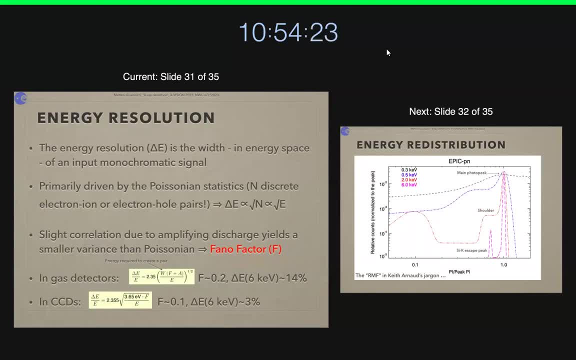 the width of the monochromatic spectrum that your detector measures. So in X-ray astronomy, you know I'm going to talk about grating, I'm going to talk about microcalorimeters, but most of the detectors we are going. 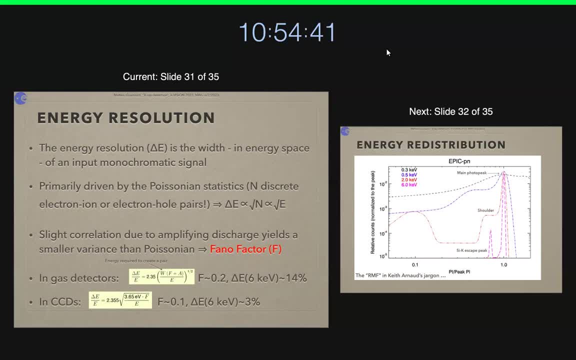 to deal with in these days. they have a relatively poor energy resolution, Which means that if I measure a monochromatic line of energy 1kV, my detector is identifying the photons corresponding to energies that are not 1kV. 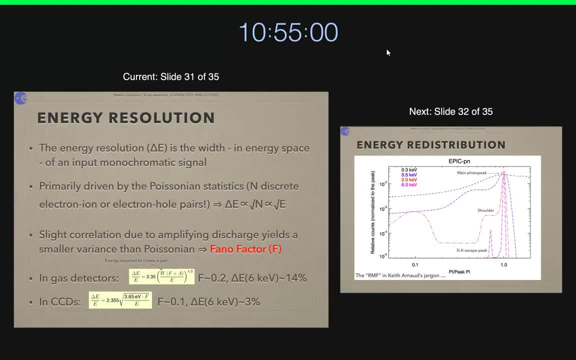 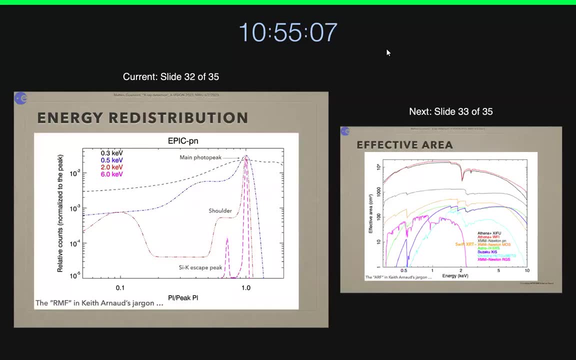 Only a small fraction of them will correspond to 1kV, Some of them will correspond to lower energies, Some of them will correspond to higher energies, And the shape of these distributions is a nightmare and is energy dependent. So this is how. 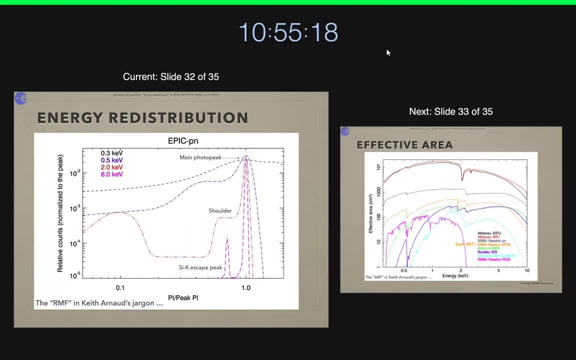 actually this is the spectrum, the conceptual spectrum, of a 1kV line observed by the EPIC-PN. Sorry, it's the conceptual spectrum of an energy, of a line at the given energy, and the energy is given by the colors. 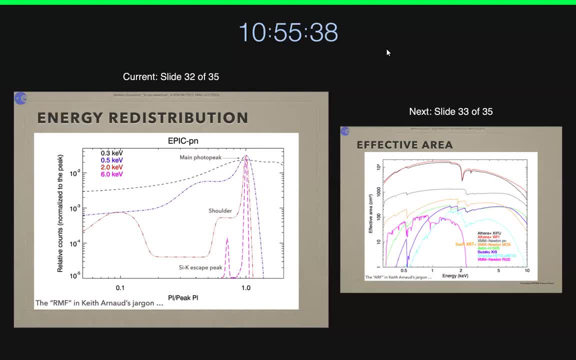 We go from 0.3kV, the black line, to 6kV, the magenta line, And on the x-axis, I just show the ratio between the channel where the line should be located, according to the theoretical relation between the number. 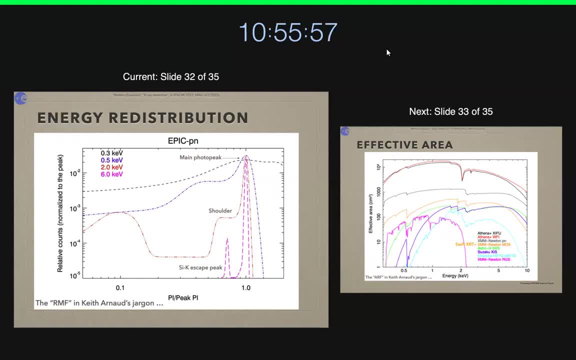 of events and the energy of incoming photons and the truly detected energy by the detector. So look at the black line, for instance, the dashed line. This is telling you that if a photon of 1kV impinges my detector, there is a not negligible 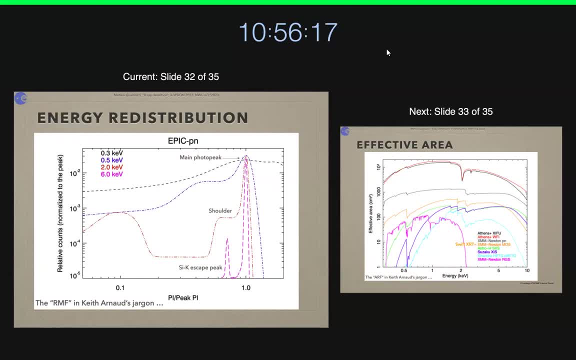 actually rather large probability that the cloud of electrons that I measure in my detector corresponds to energy of half 0.5, 20% to 0.2,, 10% to 0.1.. And you have to imagine each resource is a continuous spectrum. 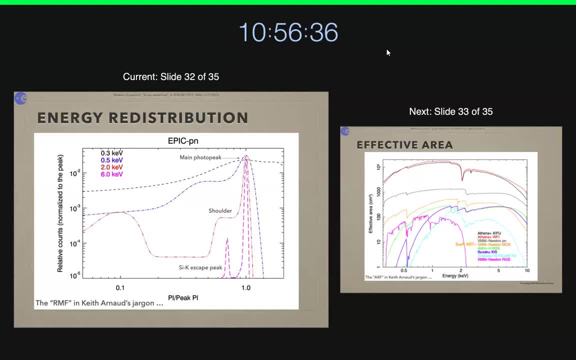 So imagine they convolve the energy of a given event, measured by the energy of the given event using the measured PI channel, knowing that you don't have a one-to-one correlation between the spectral channel in your detector and the incoming energy. It's a nightmare, but there are. 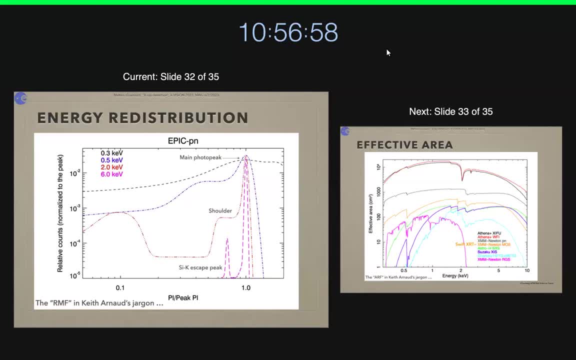 people who have done the job for you and you can use what they have done. This is the concept of redistribution, matrix phi, which is very common in astronomy, and you will get familiar with it at the latest in my presentation on X-ray spectral analysis tomorrow. 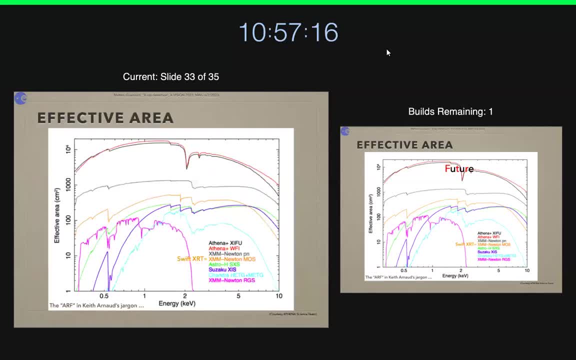 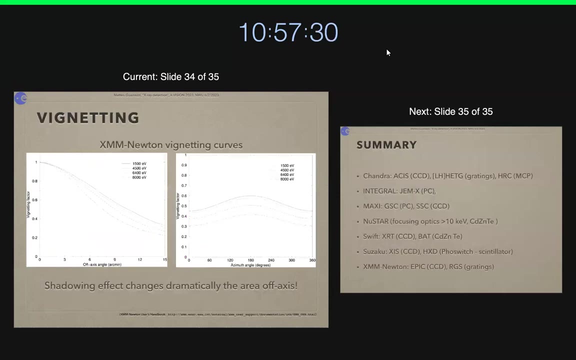 but probably earlier with Sumil later today. I've already showed you the effective area. Just to remind you, effective area is the collecting power of your telescope plus detector as a function of energy. But another aspect that is for you important is to work with both XML. 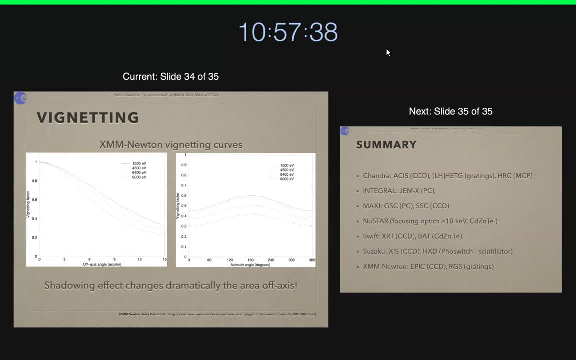 and NISTAR data. The effective area is not the same over the field of view. There is a sort of shadowing effect, self-shadowing effect in all X-ray optical systems, making that the effective area of axis far from the position of the optical axis. 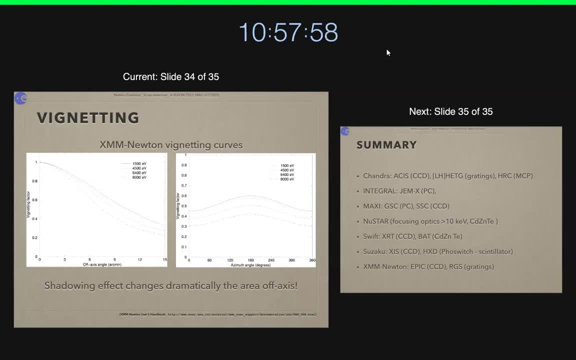 is lower than at the center. So if you look at sources of axis, the real effective area is, in the case of XMM, for instance, at the distance of 15 Arminus from the center, is less than 50% than the effective area on that. 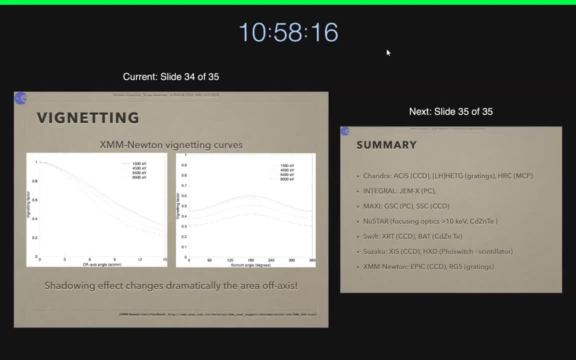 So when you work of axis you have several problems. You get less photons, you have a much more distorting imaging profile. I'm not discouraging you from working with of axis sources, but if you work with of axis sources or with extended sources, 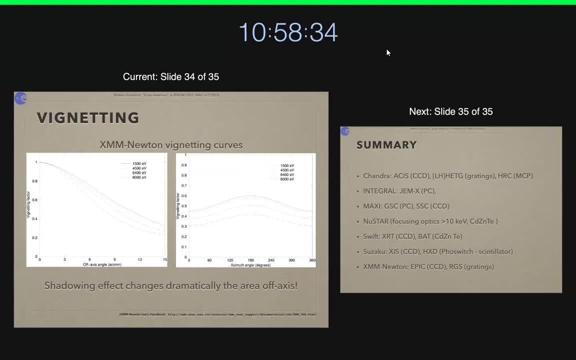 very extended sources, your life will be more exciting. I don't want to say more challenging, I say more exciting. That's all I wanted to say for today. So I thank you for your attention and I'm glad to take any questions you may have. 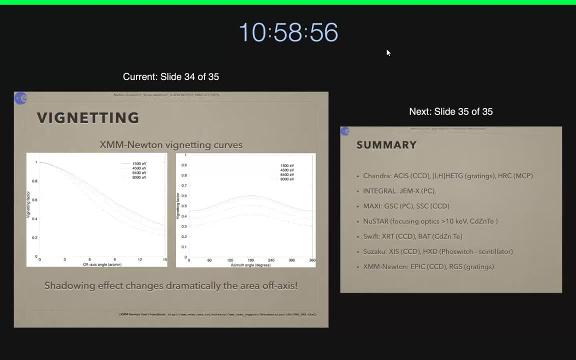 Yes, first of all, the question is: many of us are not X-ray astronomers, so we are not all aware of the. that's a very good point. normally, I always explain them. 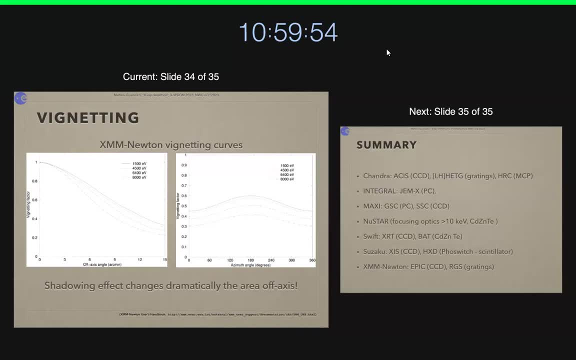 but I think you're right. it may be an example of, and because EPIC is one of the instruments on board with, and of course this comes after, to be logical, to talk about EPIC after the presentation on it's a very good point. I gave this presentation once. 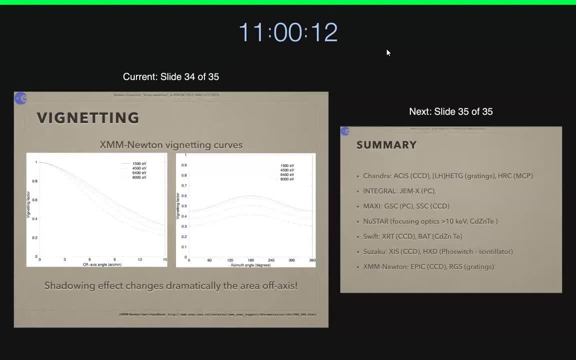 and this point was not made so I didn't correct it, but I reckon it's an issue and I thank you for your attention. in a specific case, EPIC is the European Open Image Encounter. it's one of the CCD instruments. is there any other shortening? 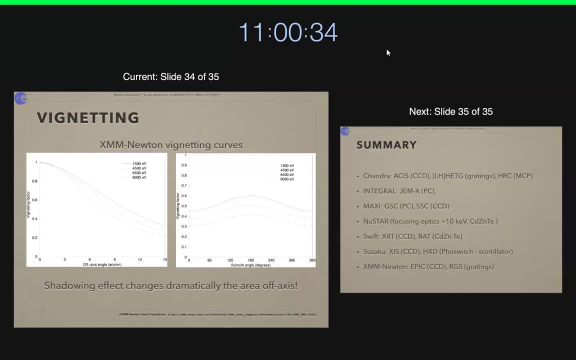 yeah, but you know, if there is anyone that I mean I've not understood anything, I mean I've not understood anything. I mean I've not understood anything unless we tell you what this means. and my last question is: I mean I've not understood anything. 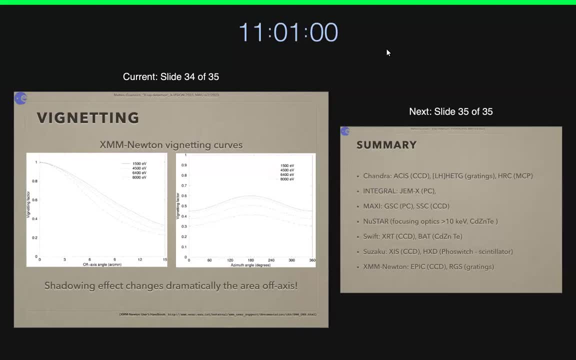 maybe if it's a, that's a number. I'm not sure the whole system is terrible. So so your question is: why? why are the three detectors redesigned to be total counting? I'm just asking: how carefully are they designed in such a way that each pixel is at least six? 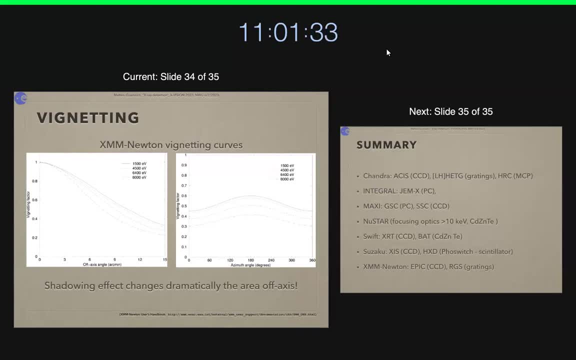 Yeah, well, you know this is. this is actually very good to have you know. the question is: why were the detectors designed in such a way to get to that one pixel gets one event? Well, they have been designed perfectly this way because knowing so, being able to associate the pixel to a given event, is very important, because it can tell you where the event happens. 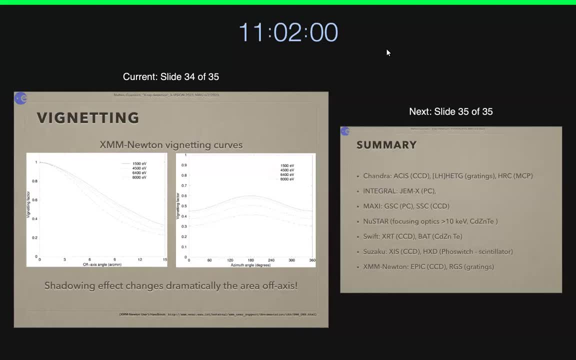 If I were there, if I were just a system. they just tell me in this volume an event happened, but I don't know where. No, it can happen in a very large area of the sky, And this doesn't help me in doing detailed spatial analysis of each of them. 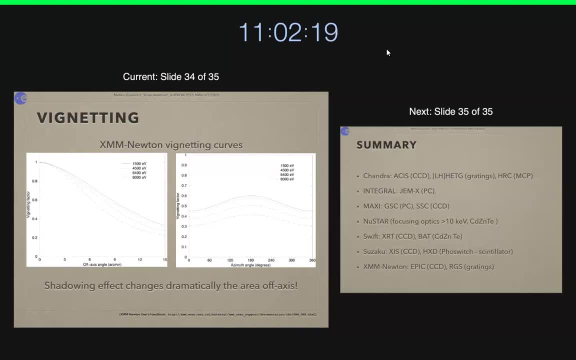 And the second reason is if I can pinpoint exactly in the array of pixels where the event happened, at that point I can highly decrease the signal to noise because the number of background events corresponding to that pixel it's much smaller than the number of background events accumulated over the whole detector. 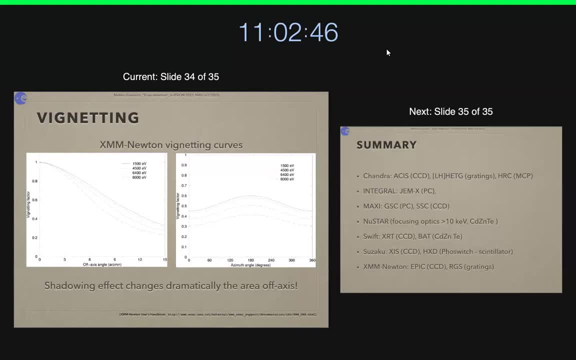 Remember, as an order of magnitude, the background scales always to the volume of the detector. So if I can give my analysis only of the background which is detected in the very small region of the detector, I can detect a much greater source. So this design is actually clever. 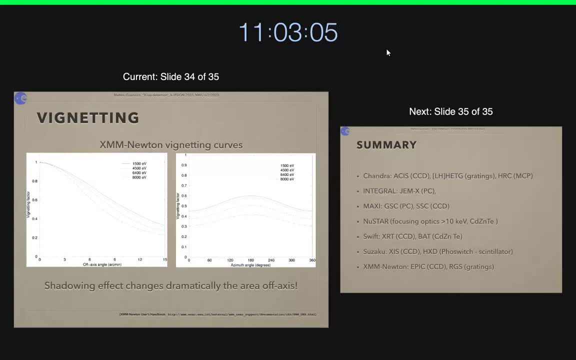 And it's designed this way in order to achieve this goal. Yeah, And that's why we have an observation, because we are having all kinds of energies and all kinds of photons. We want the camera to be able to detect the photons with low energy, but also with high energy. 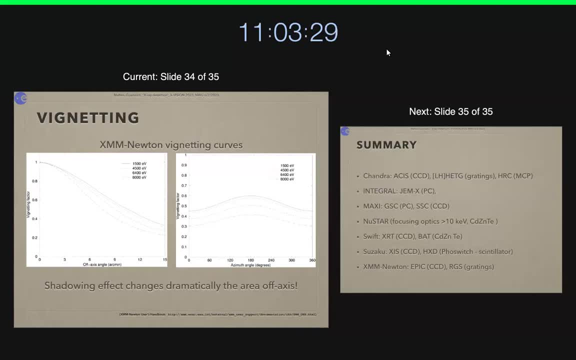 Maybe it can take 30 seconds. Yeah, So I wanted to know what that is. Yeah, So this is an area, but it's an area which is the product of a geometrical area, of the mirror, times, a certain number of factors which represent the efficiency of detection of your telescope and of your detector. 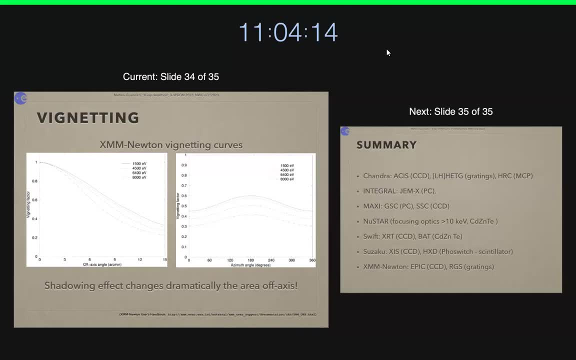 For instance, not all the photons impinging your telescope's given energy are detected, because only those that are only fractionally related to the reflectivity of the material, Which is the reflecting circle of the telescope, are actually going to the focal plane And in the focal plane, the detectors. not all the photons reaching the detector. they are revealed, they are detected by the instrument. 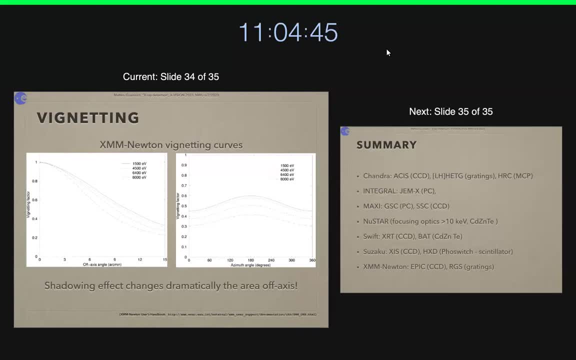 Some of them are lost. So when we take the geometric area of the mirror in centimeters squared, Can you explain the geometric area? Geometric area is really. you know, Yeah, It is a square, It is a circle. Radius squared times five. 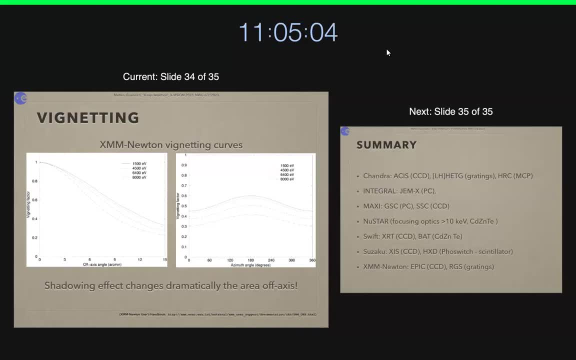 That's the geometric area of the mirror. Then I can multiply for a series of factors comprised between zero and one, And this multiplication leads eventually to the definition of effective area. So I think an energy is the geometrical area of the mirror in the Euclidean sense. 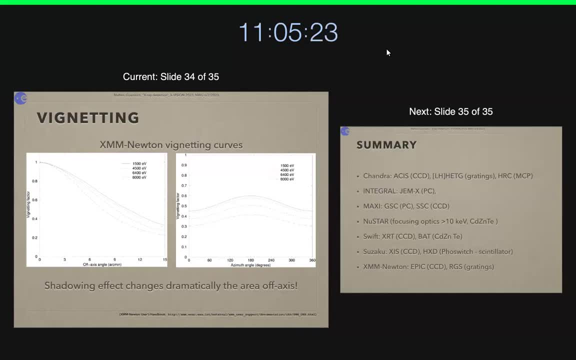 The third energy times, the efficiency of the telescope And the efficiency of the detector. The efficiency of the detector includes the quantum efficiency, Includes the filter transmission, Includes the dead time effect, Includes lots of different things. Some of them will be explicitly dealt with in the data analysis sector. 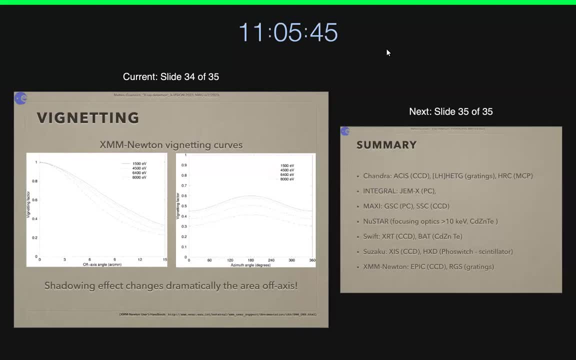 Because you need to know about these effects, But some of them you don't really need to know. You just have the effective area at the end, Which is the product of everything else. You just use it. But that's the meaning, Okay. 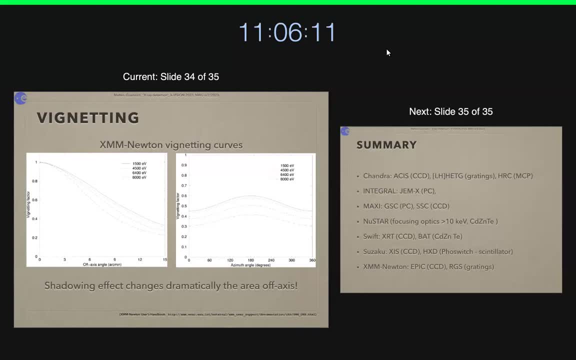 Calibration means what We calibrate, We don't calibrate, You don't calibrate, You don't calibrate, Yeah, You don't calibrate, Yeah, The way, Okay. Calibration is in itself, It's in other forms of. 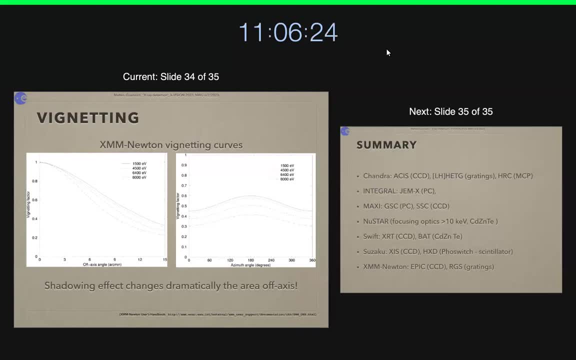 And you know, once again is the right person to ask, Because it's coordinating a group of several types of science And it's primarily. But in a nutshell, The good news for you is that in 99.9% of the cases, 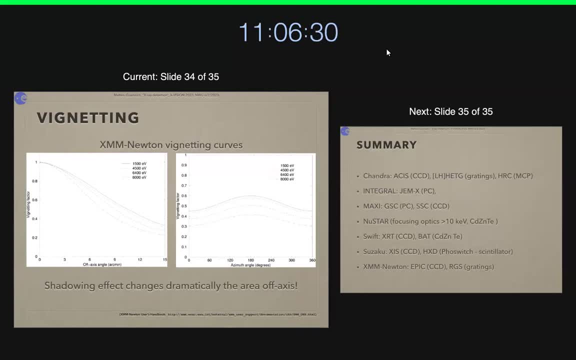 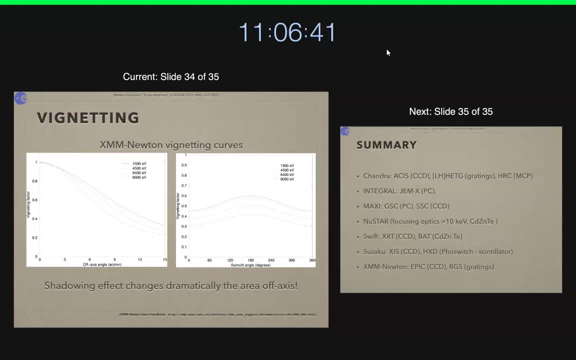 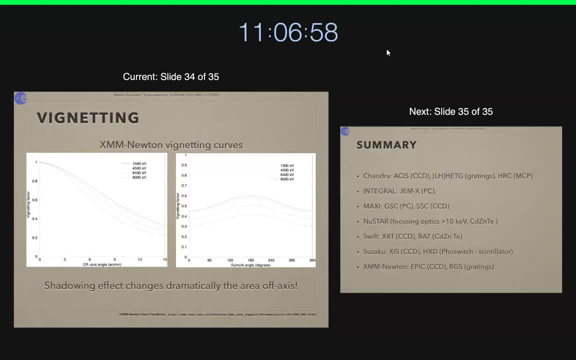 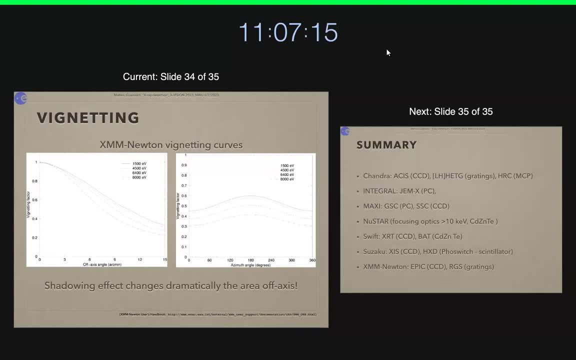 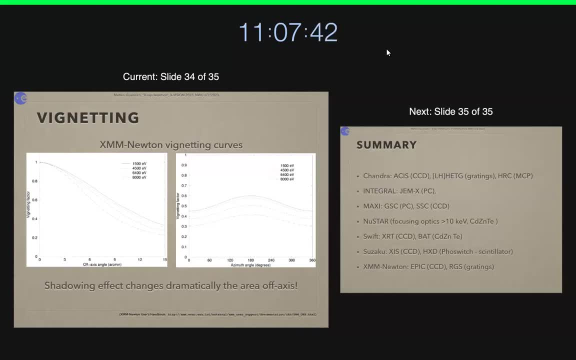 Yeah, I was just interested in comparing optical CCDs and X-ray CCDs, where, of course, in optical CCDs the amount of detection is only really dependent on flux in the optical, not the energy, quite different to the X-rays. 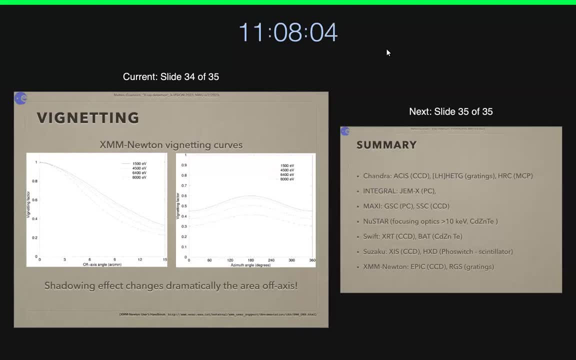 And of course, in optical CCDs we typically back-aluminate and thin them, use different sort of resistors And to promote the sort of proficiency of low-energy optical photons In the case of X-rays. obviously, if you just illuminated one of those CCDs, the X-rays 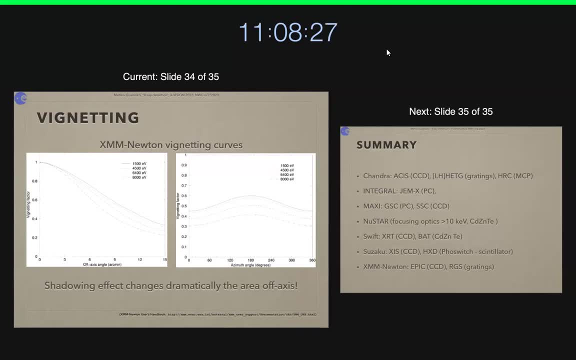 would just go straight through the device. So I'm sort of interested in knowing how the CCDs are developed for X-rays by the same companies, right? So it's specific to X-rays. It depends They are. some of them are produced by companies. 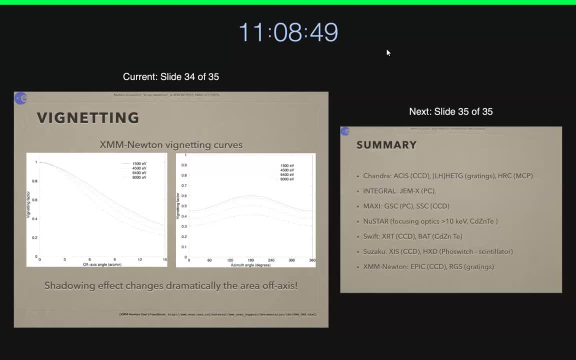 Some of them are developed in our research. In fact, for instance, the PNCCDs, they are produced by a company which is actually a spin-off of a laboratory at MP, So now it's a company. but eventually all the people that are the people that made the 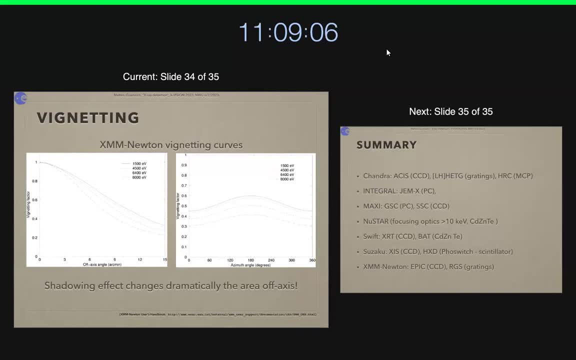 work in MP. I think the reason why it is a company is just because it's probably more Yeah, Yeah, It's a managing. the managing concept is more cost effective to run a thing like this as a company rather than as a as a as an institute, a research institute. 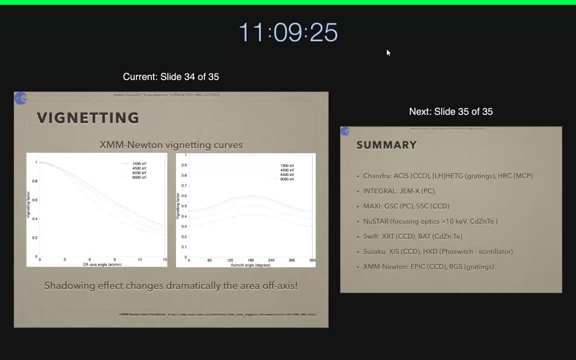 But for instance, in Japan, the CCDs on Japanese mission. they are created by the no, no, yeah, So it's a private undertaking. So there's something different that has to happen between the two. Yeah, Yeah, Yeah. 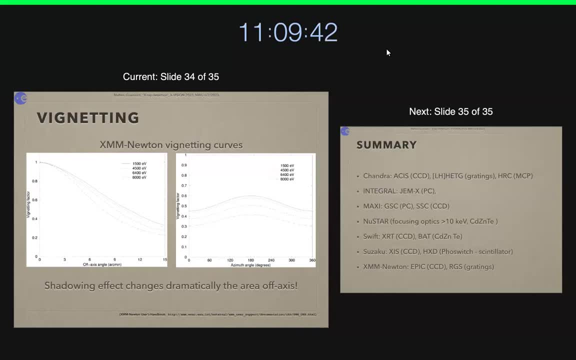 Yeah, Yeah, Uh. And just one follow-up is: what is the um charge transfer efficiency of the X-ray CCDs Cause in the optical we used to what we call 4x9s, It's 99 indirect. 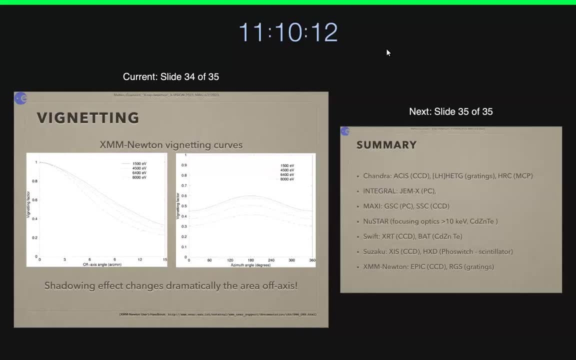 Oh, or nine, nine, nine, nine, CTV is it is? it's a no, it's in each step is very low. it's a 10 to the minus five, if I remember. yeah, but we have a larger raise of pieces, so, and we have many photons, so we have many electrons, so eventually, the number of electrons that we 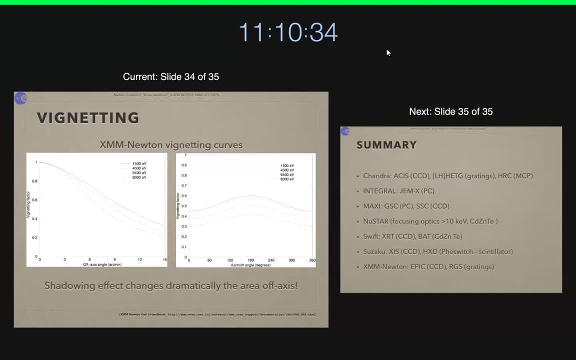 use when we integrate over the whole globe of columns. it's not an ingredient, it's an effect. it's an effect at the readout node, that is, of a few percent in case of some end. so you know you need to calibrate it if you want to achieve that. you know we want to achieve. 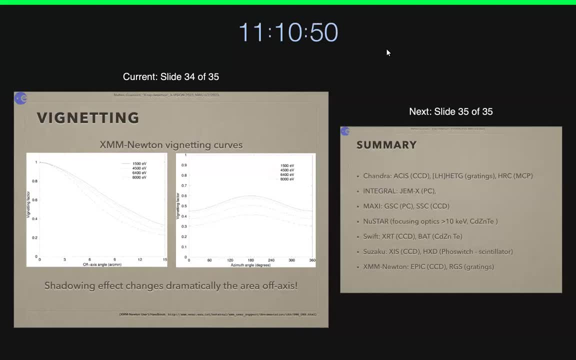 accuracy of the end of the construction, which is of the order of 10 ed. in principle. so it's 10 ed are three electrons, so you can easily use much more than three electrons. so we are perfectly calibrated and it's energy dependent- all kinds of things. 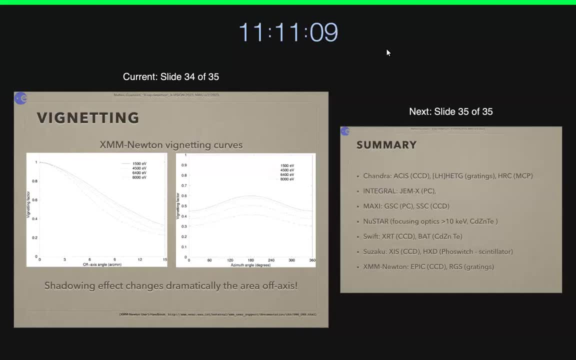 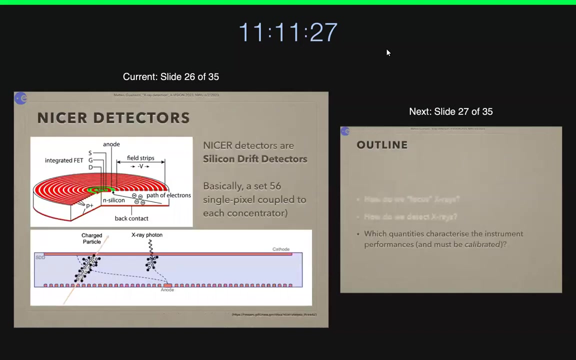 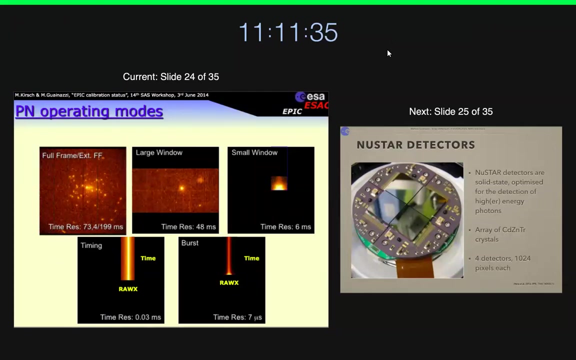 uh, yeah, it depends, of course, on which one. so for the, I think I have the numbers here. for instance, that's an example, for just an illustrative example, for already a CCD on board, so I don't use uh shortening, uh, so in the largest frame. so 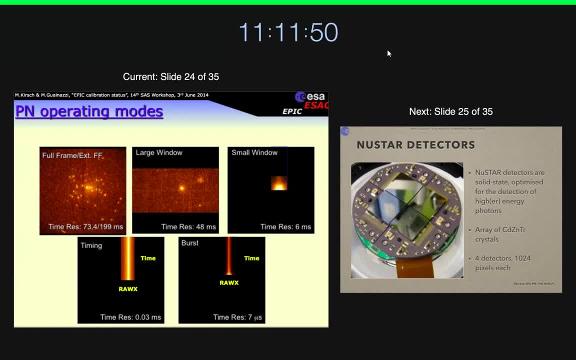 the slowest mode is still the order of between 70 and 100 milliseconds and in the timing mode which is the fastest, is a seven microseconds. uh, for the other CCD camera on board- it's a new gun, it's the total similar ballpark pretty soon. no start timing solution. it's not microseconds. 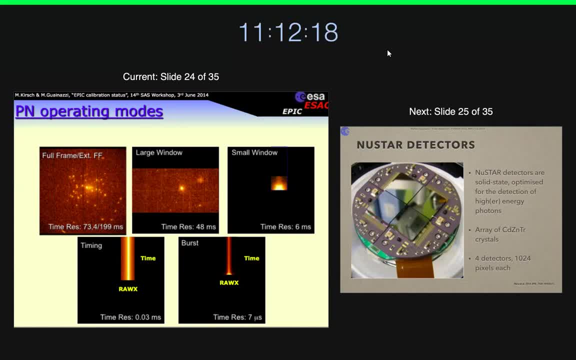 yeah, ah no, no, no, no, sorry, this is just that. you know, this is just the time you can be run without the next. but then you know the observation, the observation, bacon eating for hundreds of hours a day. you just accumulate the day. So essentially is either probably: 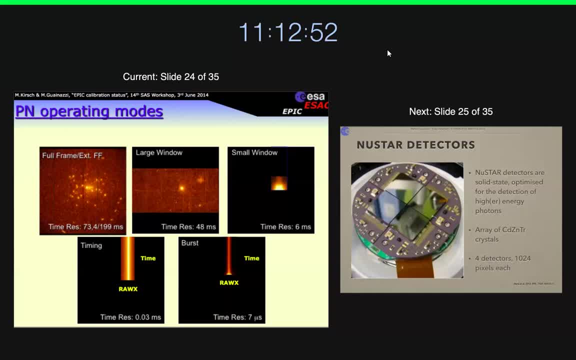 going to show me later- Basically all the missions. I think this is applied to all the missions that we work with. We work with events, So for each event we have one row in the large table which contains all the problems, the patient, the.